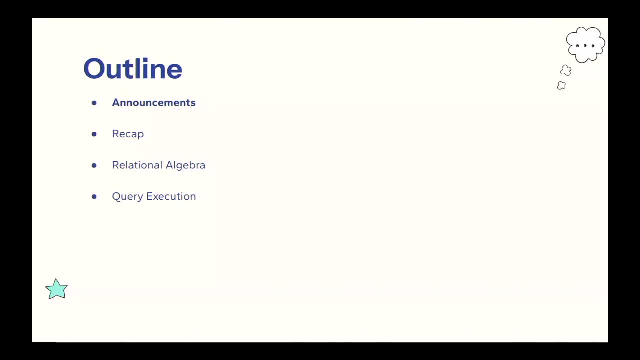 And after that we will learn two important topics: relational algebra and query execution. So the first announcement is that we don't have any quiz this week. However, you will have your quiz six due by next Friday and that is your last quiz. 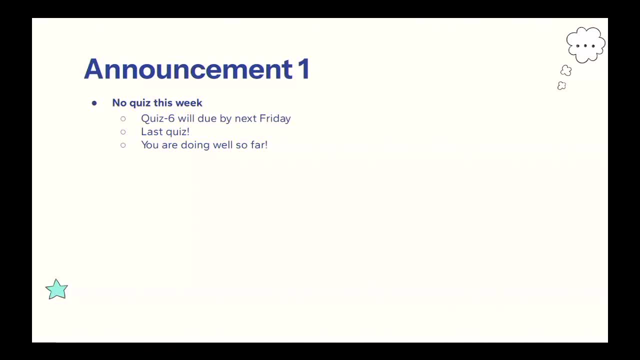 And as for the scores of the quiz, you are doing pretty well so far and the average score is is a little bit higher than previous terms For. the second announcement is about assignment two, So we have released the specifications for the first two questions. 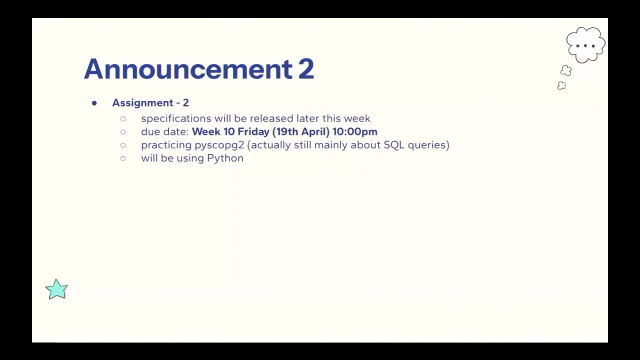 and we are finalizing the last three of them and the due date is by the Friday next week And and you should, you should submit your special considerations early, as early as possible, and you should submit your ELP extension request 24 hours before the due date. 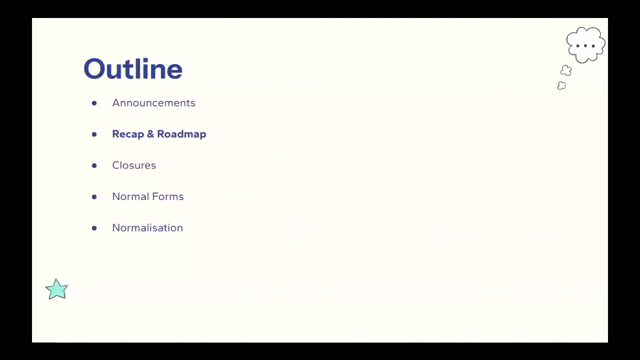 And that's all about the announcements. Let's have a quick recap and have a look at the roadmap. So in our last lecture, we have learned the actual usage of functional dependencies and we have learned several important concepts. The first one is a closure. 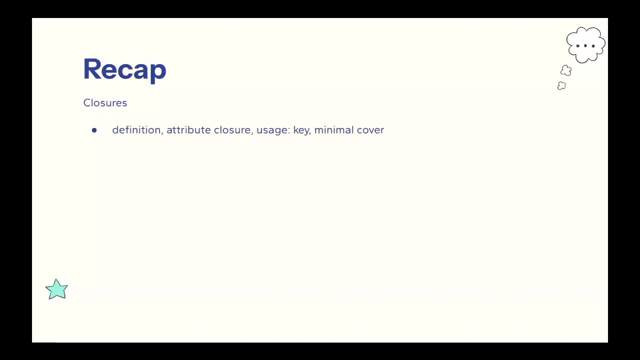 So can you still remember the definition of closures? So what is the definition here for closure? Given a set of functional dependencies, what is the closure for this? The closure for a set of functional dependencies is the set of functional dependencies that could be derived based on this set of functional dependencies. 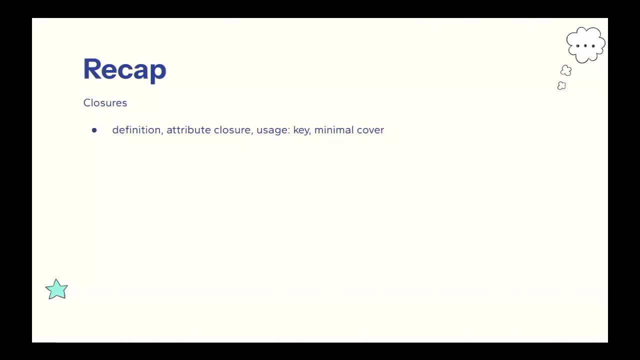 So that is the definition of closure. However, the closure for functional dependencies is often very, very large, and it is impractical to be used for many algorithms, So So, instead of using functional dependency closures, we use attribute closures, And 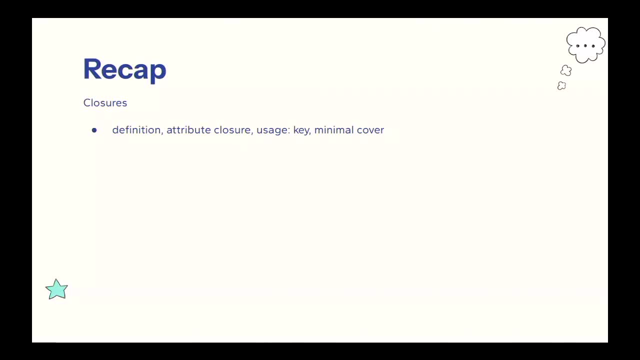 And do you remember how to calculate the attribute closure? You don't need to worry if you can't remember the exact algorithm, because I will show you our plan next to help you to memorize all these concepts: And And And. the usage of closure is often related to determining keys. 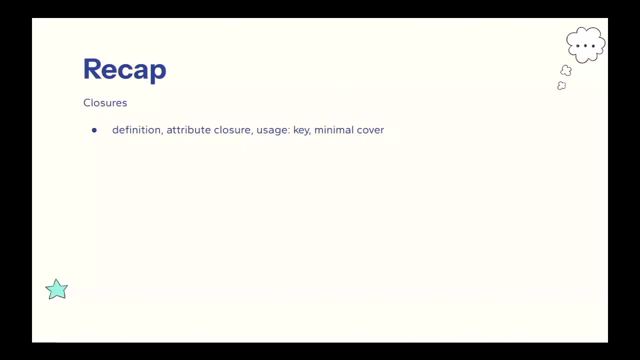 because the closure for keys can cover all the attributes of a relation, So that's the usage of closures. And another concept related to closure is minimum cover. It is the smallest complete set of It is the smallest complete set of It is the smallest complete set of functional dependencies. 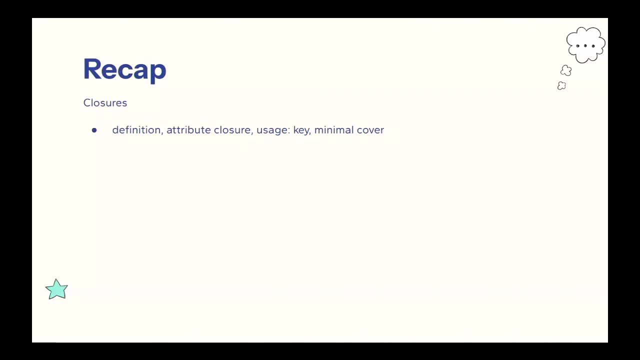 So that's the definition of minimum cover. And the second key concept we learned in our last lecture is called normal forms. So the most commonly used normal forms are the third normal form and the BCNF. So do you remember which one is the third normal form? 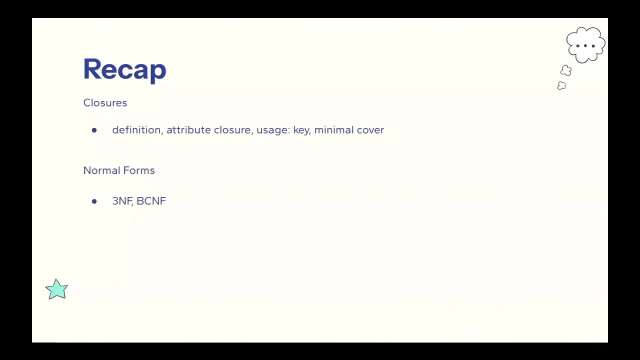 And which one is Has less redundancies, Which one we will use as less redundancy, BCNF actually, And- And I hope you can remember the restrictions of these two restrictions or normal forms. So this is, This is actually the. 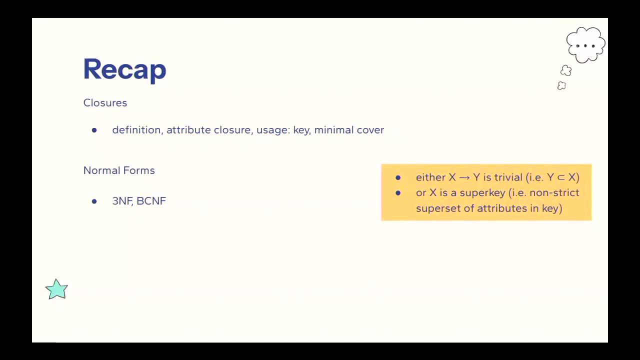 The restriction for the functional dependencies Required by BCNF, And these are the restrictions required by the third NF. As you can see, it has one more allowed pattern here. So third NF is a little bit less strict than BCNF, So it allows more redundancy. 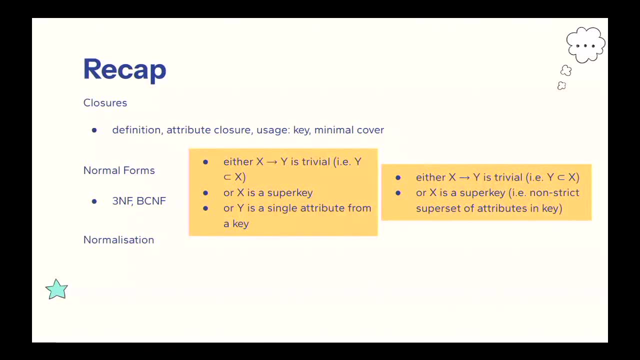 I'm talking about normal forms. We have learned the process of normalization And we have learned some algorithms for calculating third NF or BCNF. So you don't have to recite. You don't have to recite the algorithm, But you have to understand how it works. 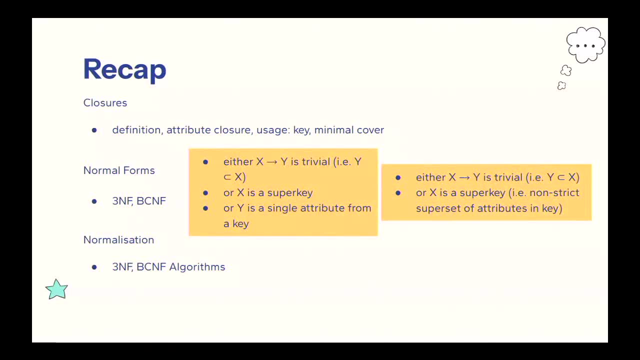 So for third NF, the algorithm starts with building reduced minimal cover Of the functional dependencies And, starting with the minimal cover, we gradually include tables into our collection Schemas, into our database schema. So that's the algorithm for third NF. 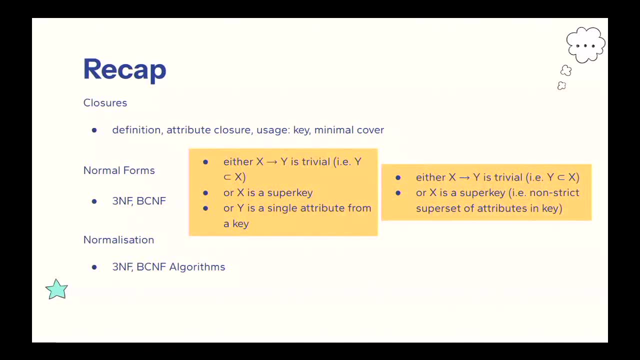 For BCNF. the algorithm is to check, To go through all the functional dependencies one by one And try to identify Whichever functional dependency that will violate the restrictions of BCNF, And then we separate tables according to the functional dependencies that could violate the restrictions here. 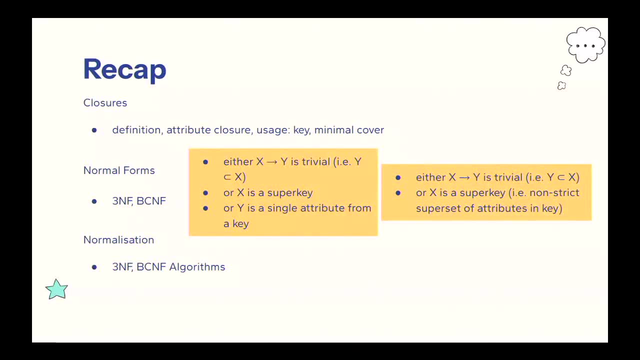 So that's the algorithm of BCNF. So our plan here is like this. So, instead of getting you overwhelmed by those algorithms- Because there are several details And it is quite lengthy, So you don't need to worry about reciting those algorithms- 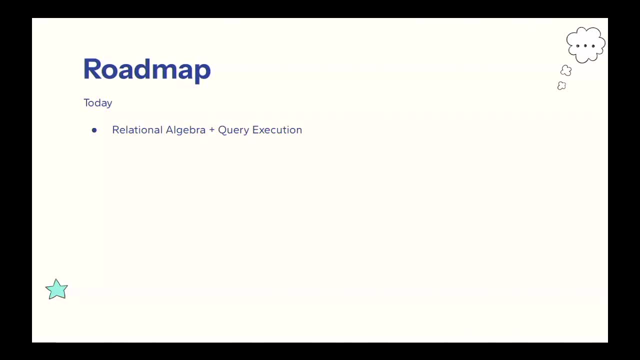 What we will do now is Our plan is: I will guide you through all the. I will give you all the concepts and all the knowledge as fast as possible, And then I will provide you more Practical examples about those algorithms In our following up lectures. 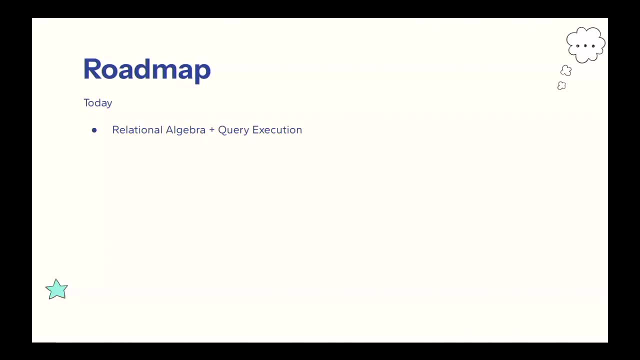 So today We are going to learn relational algebra Plus Query execution And on Thursday We will learn performance tuning, Transactions, Serializability And More examples on the theoretical concepts I don't want you to recite. 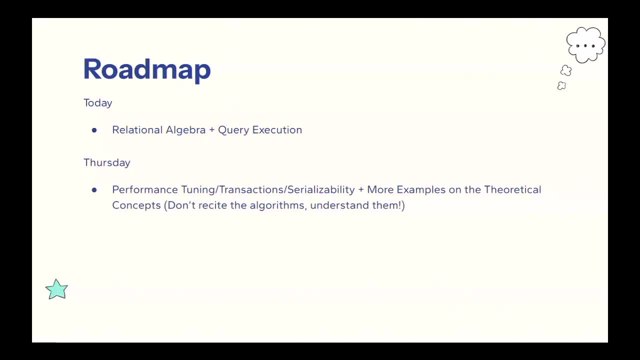 Those algorithms Instead, I wish you could understand them So. So I will try to spare some time To go through more examples for those algorithms For you to understand how they work. So In the next week I will. 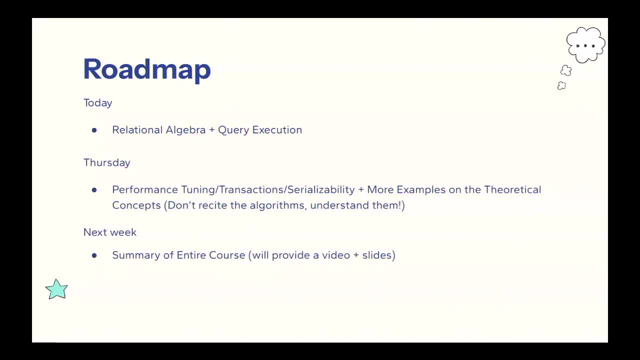 I will be out for a conference, And, But I will provide you a summary of the entire course With a video and some slides. So that's our roadmap, And And now let's jump into the main content today. So the first topic we are going to learn today is: 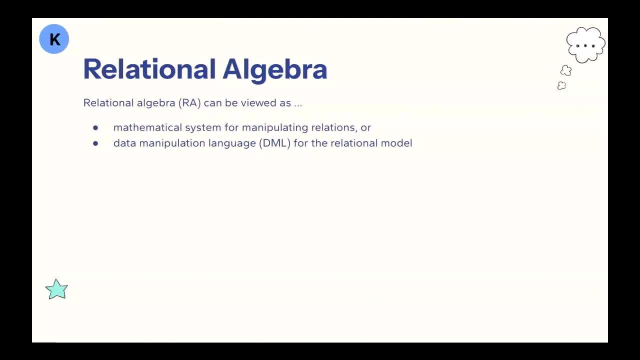 Relational algebra. So relational algebra can be viewed as The mathematical system for manipulating relations, Or It's like the data manipulation language For the relational models. So So In relational algebra it consists of Operands, Operator. 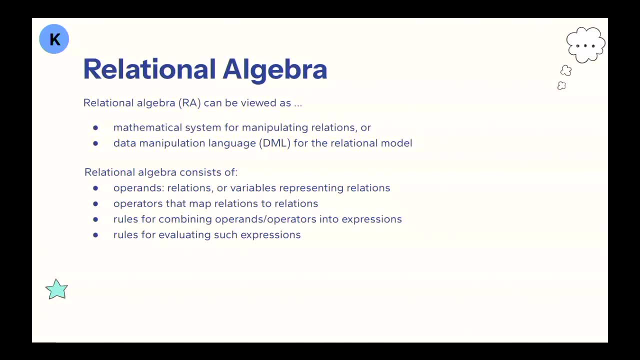 And rules of combining Operands and operators into expressions And rules for evaluating these expressions. So why it is important for us to learn Relational algebra Is because It forms the basis of The DBMS implementation. So In our previous lectures, 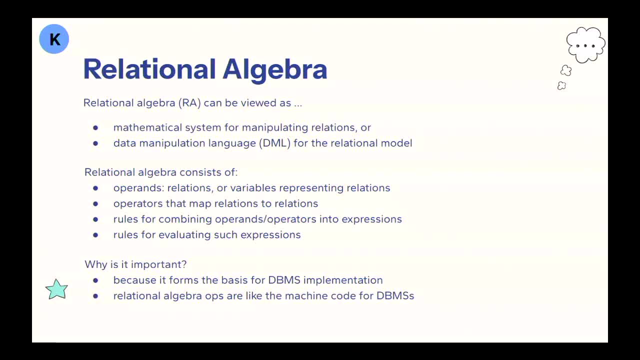 What we have learned is from the User's point of view. We learned how to design databases, Schemas, We learned how to, We learned how to use SQL And we learned how to use programming language To interact with SQL, To interact with DBMS. 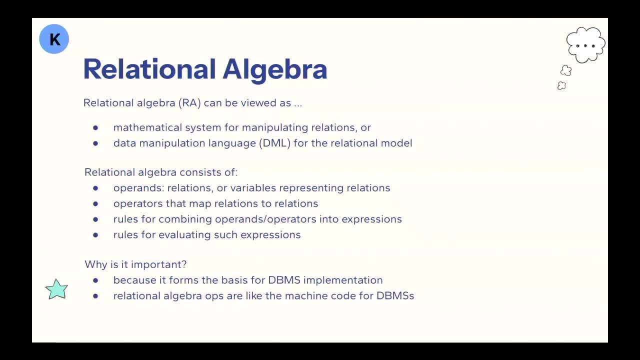 But we didn't learn from the designer Or developer of the DBMS, So Point of view. So, So what we are going to learn now is The mechanism of DBMS. So, So, this is So, this is. 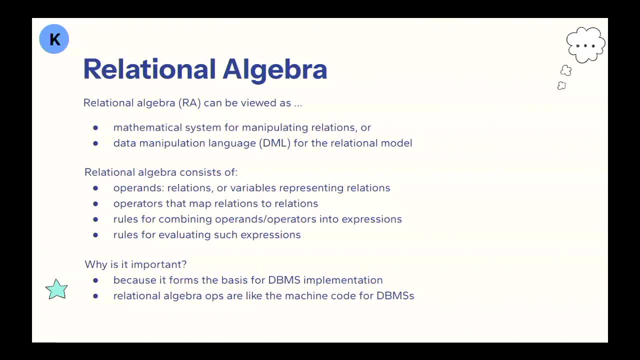 Why we need to learn relational algebra. And The second reason here is Relational algebra operations Are like The machine code for DBMS, So instead of executing the queries directly, It actually translates the queries into some kind of Relational algebra operations. 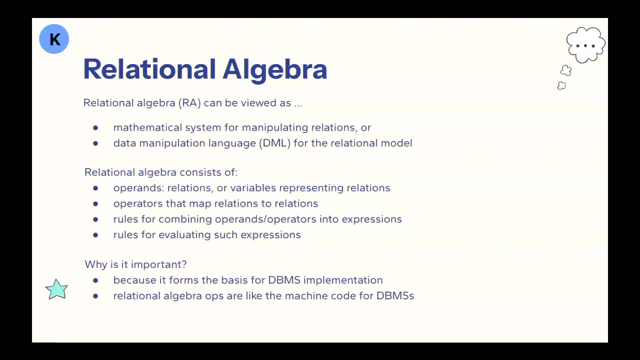 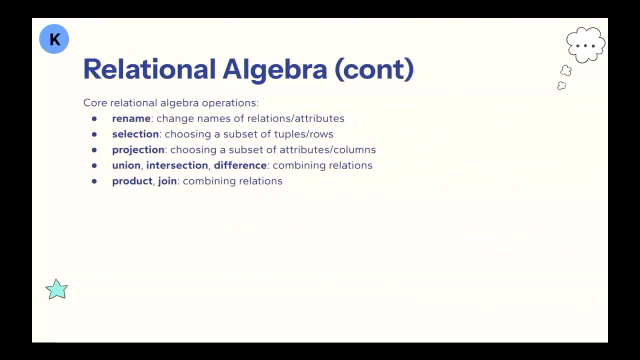 And with these, And what the DBMS actually executes Is A sequence of these Relational algebra operations. So that's why we need to learn it: And, And, And, And. most of you may expect That you are not going to. 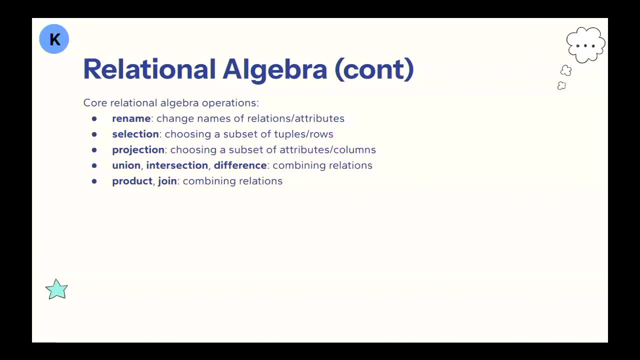 Join a database company to design DBMS, And most of you will only Be using it in the future. But why we are still learning this Is because if you know the mechanism of DBMS, You can leverage this knowledge To optimize the queries. 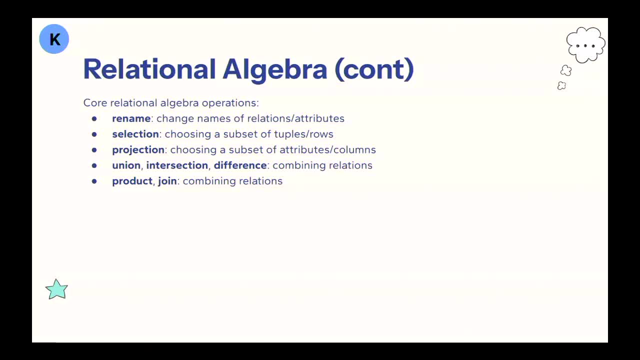 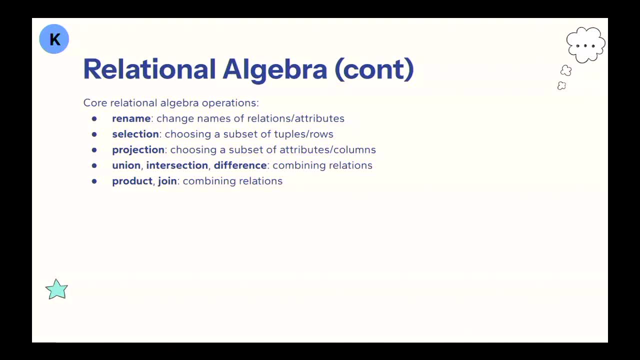 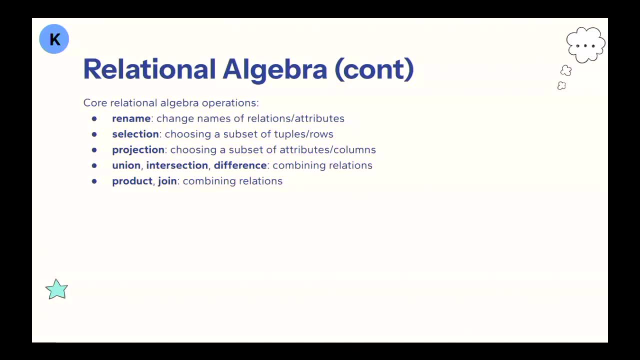 And in order to learn the mechanism of how DBMS work, we need to learn the so-called machine code for DBMS, And that is relational algebra operations. So you may encounter a lot of concepts similar to what you have learned for SQL in today's lecture. 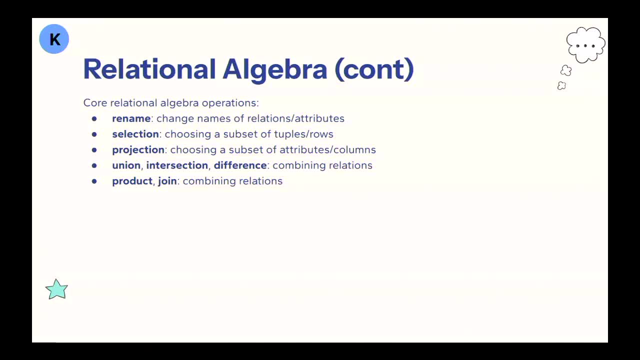 And let's go through the details. So the core relational algebra operations we are going to learn are rename, which is used to change the names of relations or attributes, And selection, which is to select a subset of rows or tuples, And projection, which is used for 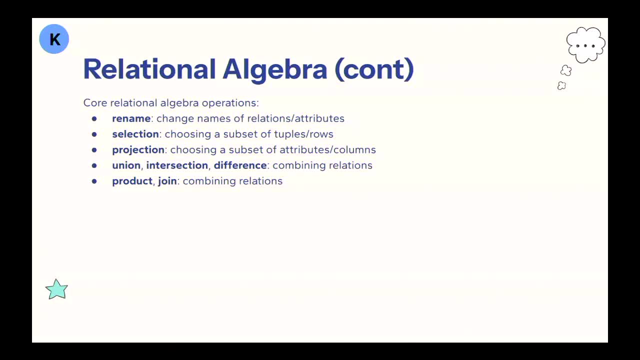 choosing a subset of attributes or calls Columns, and we are also going to learn some set operators like union, intersection or difference, which is used to combine relations, And we are also going to learn product and join, which are used to combine relations as well. 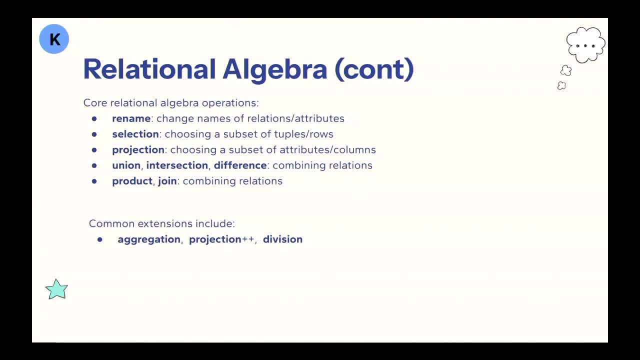 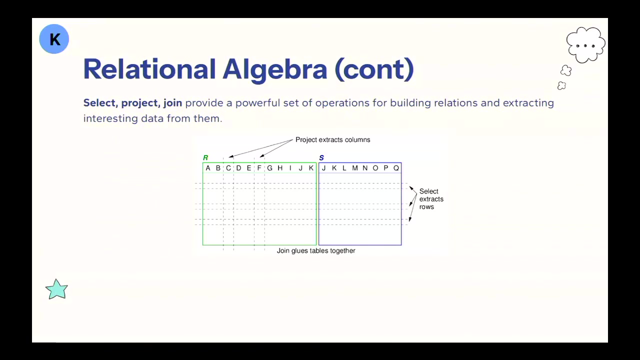 And some common extensions for relational algebra are aggregation, projection++ or division. So we are also going to learn division today, But we are now learning the mechanisms of aggregation and projection++. So let's remember the concepts of. so let's have a quick overview of what these options will do. 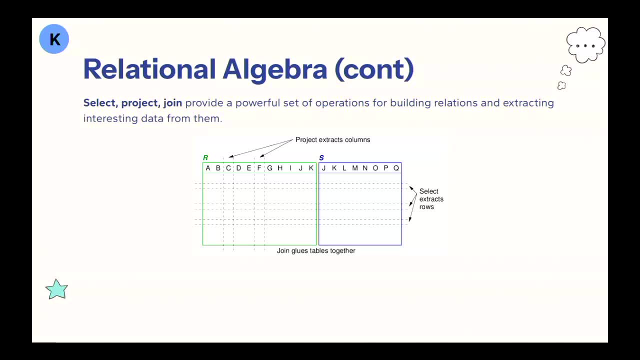 So, first for select, it actually helps us to extract rows or tuples from a given table, And project is used to extract attributes or columns And, as you can see, with project and select we can get the exact piece of data we would like to retrieve. 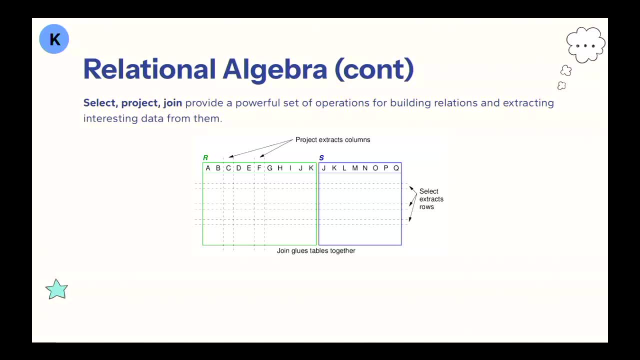 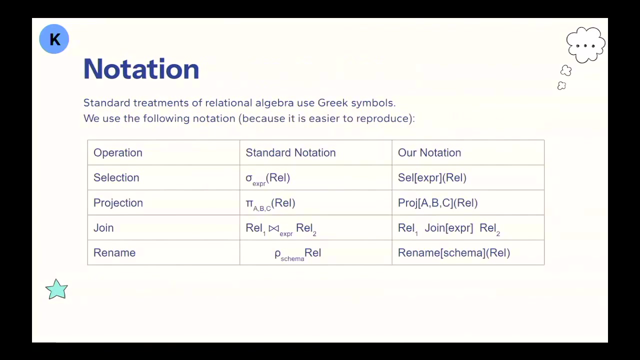 For join. join is used to combine different tables into a larger table. So that's an overview of that, these operations and- and we will also learn some set operators, set operations and renaming to make this algebra complete. So here are the notations we 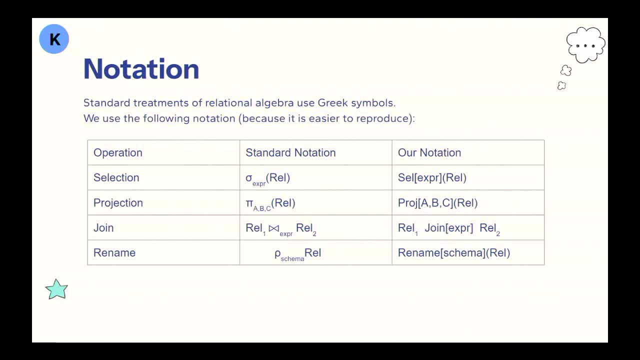 are going to use here. So so, formally, these relational algebra is using some Greek symbols that for. for readability, let's use the notation like this: So so, instead of using the Greek symbol here, we will just use select to represent select, project to represent project, join to represent join. I believe you have. 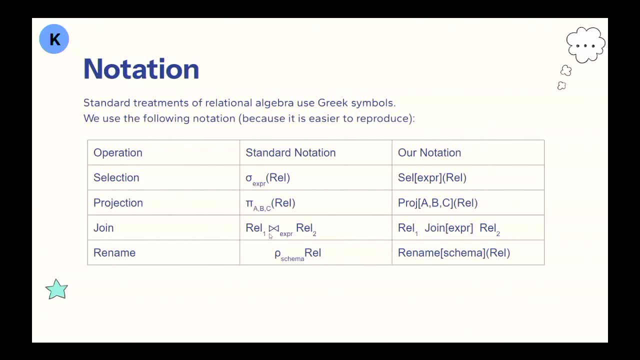 encountered this symbol in the last lecture- and rename. we just use the keyword rename. So let's use the following notations here in our slides. And for other operations we adopt the standard notation. So that's, for example, for set operations, we just use the symbols used for for those set. 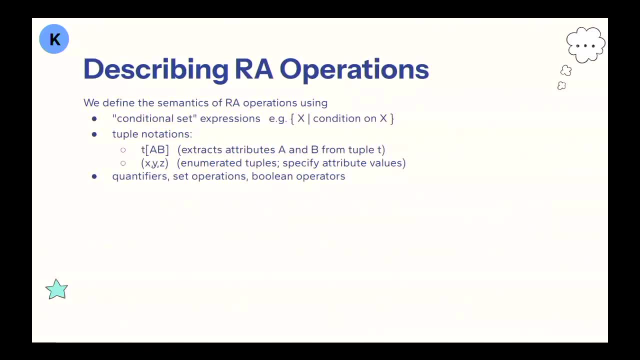 operations. So so, so in in our, in the following slides, this is how we are going to describe these operations. So we define the mechanism of operations using the conditional set expressions, because these operations will produce as sets of tuples or sets of rows, and most of them. 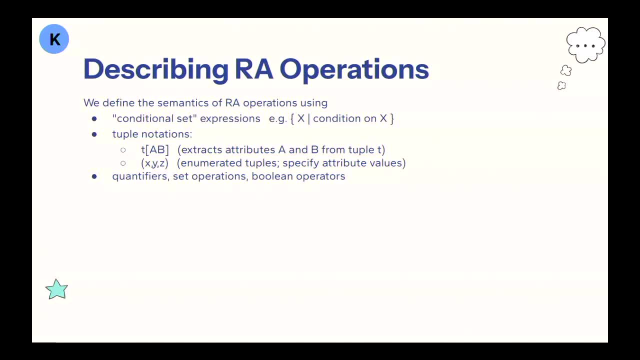 most of them will produce as sets. So this is the notation for for writing a set of values for filling certain condition And for tuple notations. here here is here are two different notations of representing tuples. So TAB representing is means the extracting attributes A and B from the 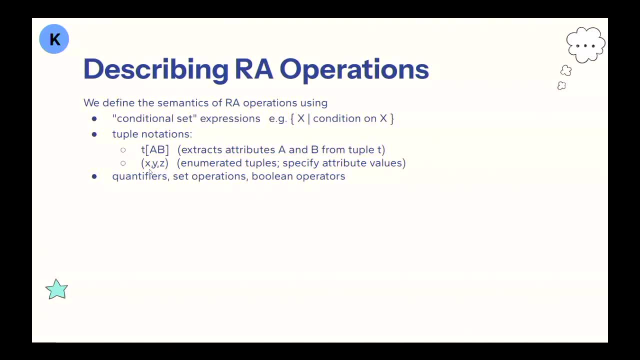 tuple T And this, this symbol, this symbol here means is a tuple with the values of x, y and z And for each operation we will also try to describe, describe how it actually works In our algorithms or plain language, But do note that the algorithm to be introduced in the following 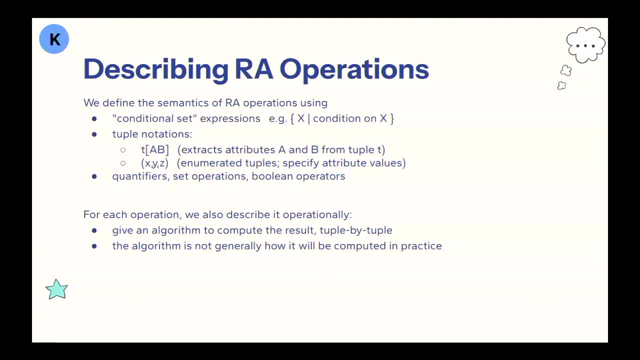 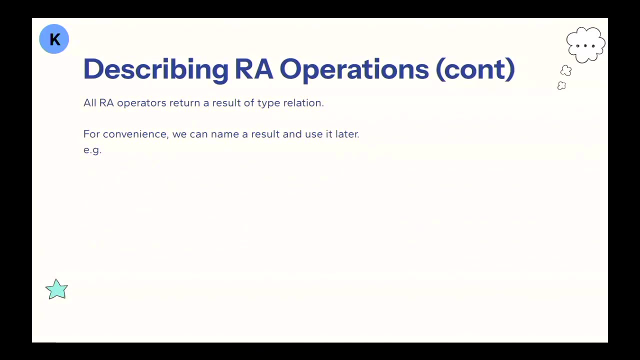 up slides may not be the actual implementation. The actual implementation that we are going representation of DBMS. so it's just to help you to understand how it works. So that's how we interpret the following slides, And here are some more information for you to take note of. 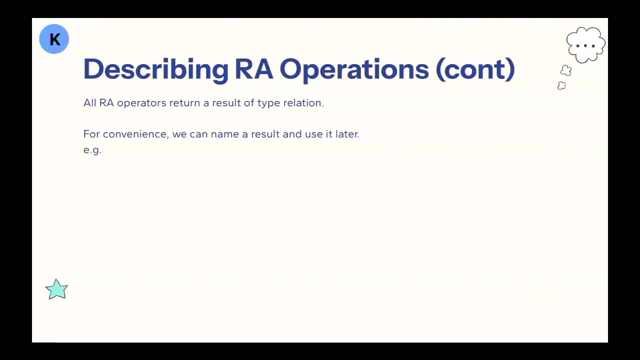 So our relational algebra operators return a result of a type relation. so it's a collection of tuples And for convenience we name the intermediate result and we can use it later. So this is an example, So we can give a name to the intermediate result of some operations. 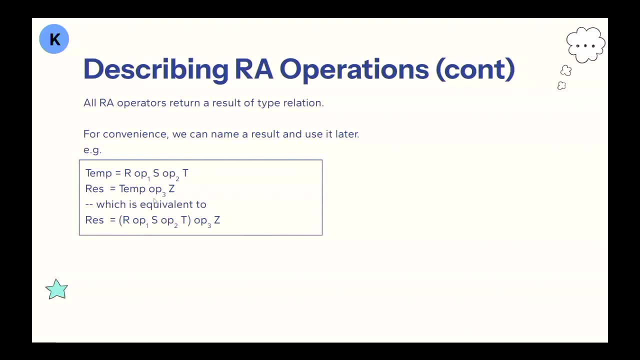 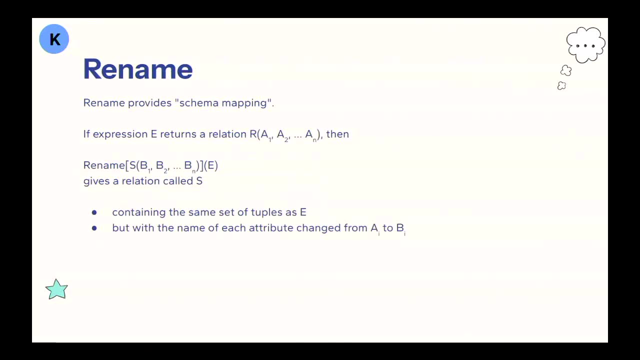 and then we can use it later. So this is just for clarity. And the first operation we are going to learn today is called rename. So it's actually very similar to how you give aliases for attribute or table names when you write an SQL query. 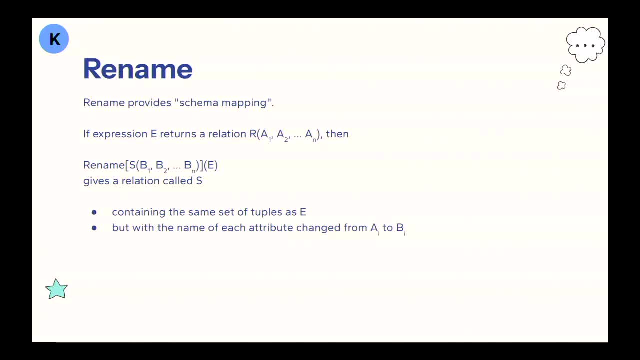 So rename provides a tool for schema mapping. So if an expression e returns a relation like this and rename will give us a relation called s, it actually contains the same set of tuples of e, And it actually, but the names are different. 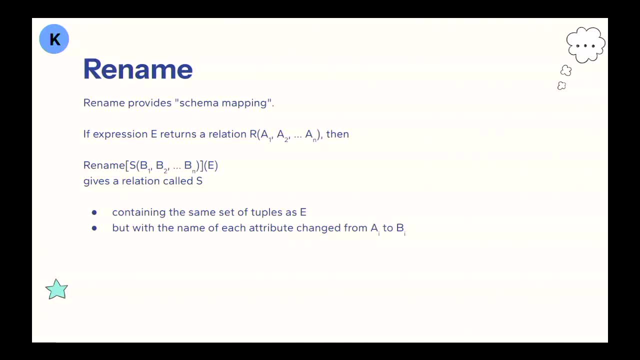 So it doesn't have any actual effect on the actual data. It's just renaming, Just giving it a name. So it is like the identity function on the contents of a relation And the only thing it changes is the schema. It doesn't affect the actual data. 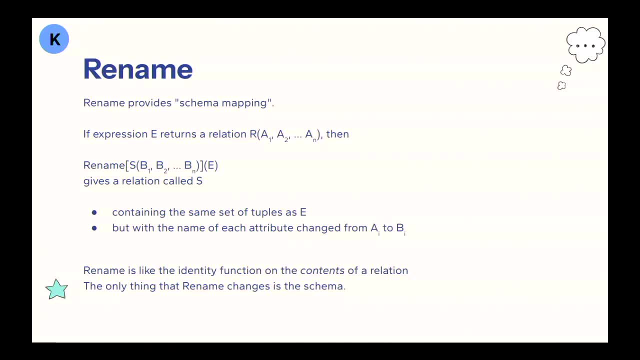 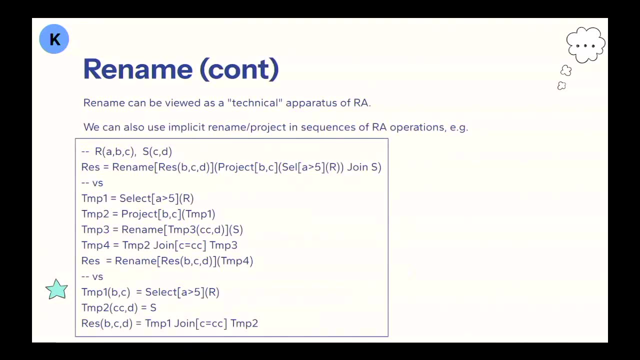 So it is just for giving the complex set of operations a new name. So So So, for example, we can actually use the rename function to rename sequences of operators instead of just one operation. As you can see here, we can. actually, these three are essentially the same. 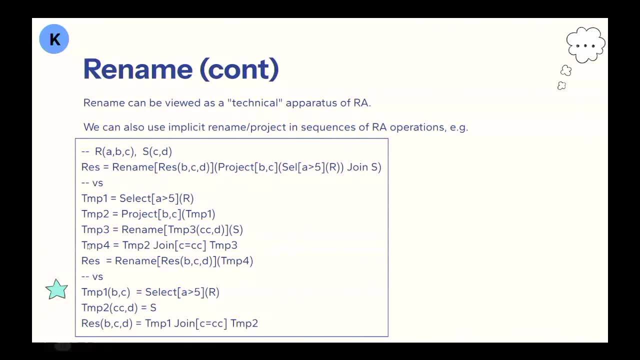 These three set of operations are essentially the same And we can use rename to rename the entire operation. So we can actually use rename to rename the entire operation, an entire sequence of operations, And we can also use rename to just rename a particular variable. 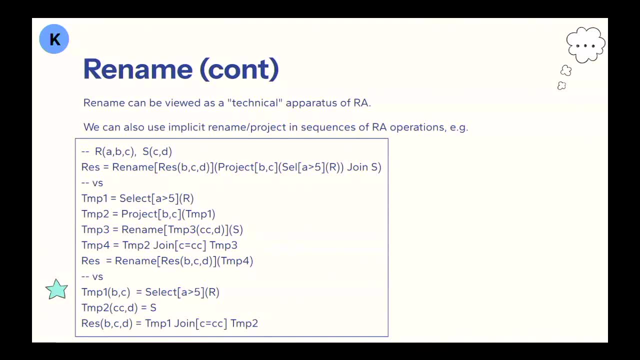 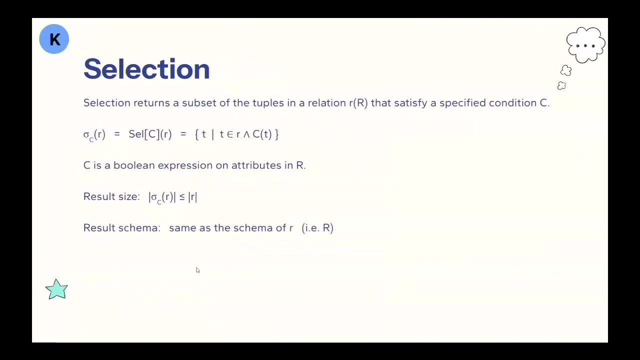 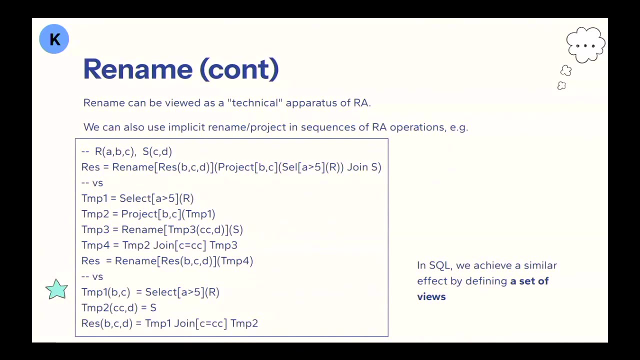 So this is the rename operation. It is actually quite straightforward And in SQL, the similar concept is, apart from using aliases- assigning aliases to attributes and tables- it is actually also similar to giving a set of views by renaming a sequence of operations. 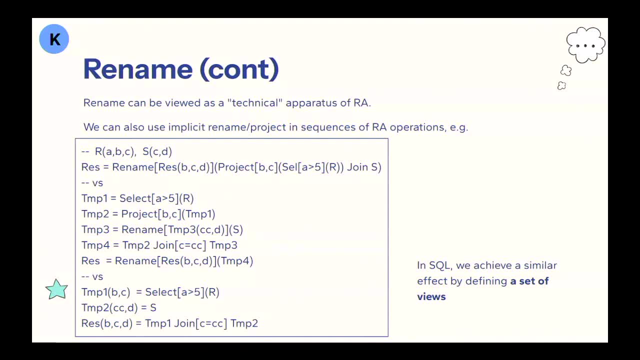 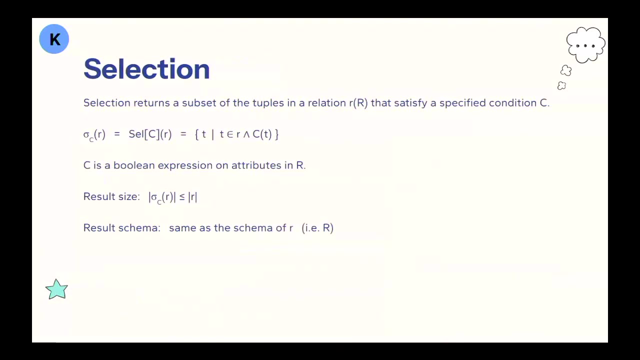 is similar to creating a set of views, So it doesn't affect the actual data, It's just to create a reference to that set of data. So that's the basics of the data. Now let's learn more about rename And the second operation we are going to learn. 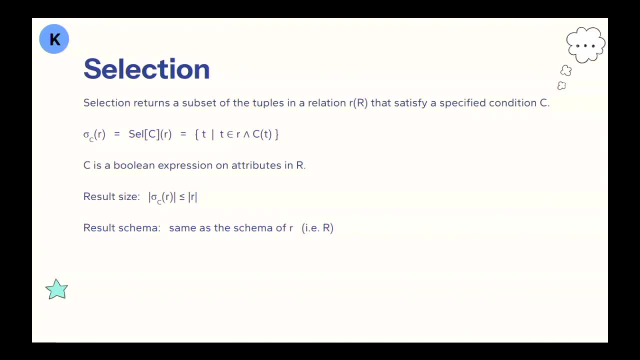 is select selection. So selection is actually a little bit different from the select keyword operation in SQL. So selection actually returns a subset of tuples in relation that satisfies a specific condition. specify the attributes to be selected to be returned. So it will just return all the attributes for given relation. 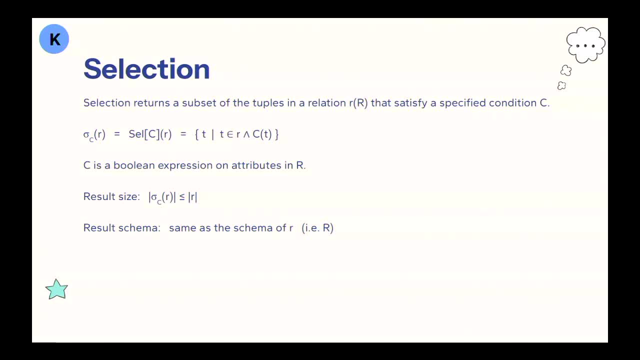 So this is select And, as you can notice here, this is the set condition, set notation for the selection operation. So how do we interpret this? is it's a set made up of elements t, such that t is from the original relation and? 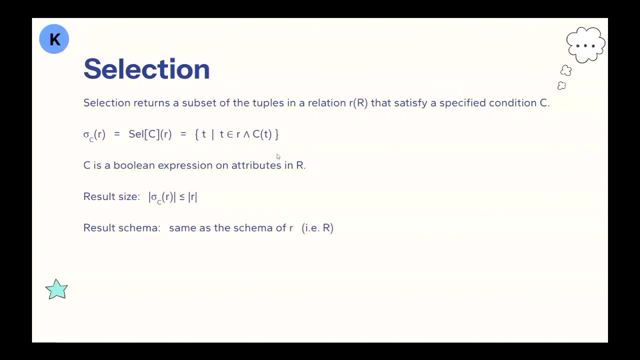 it can fulfill the condition c. So this is, this is the definition of selection And the result: size, as you may notice, is always smaller than or equal to the original relation, Because if we select everything, the size would be equal to the original relation. 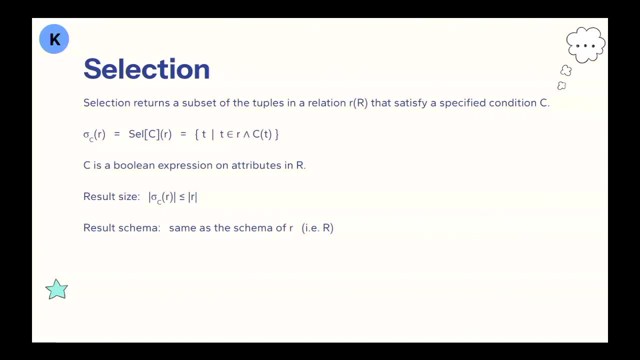 And otherwise it's smaller than the original relation And the result schema- the attributes- is the same as the schema of R. So with select we don't here in relational algebra we don't specify the attributes to be selected, So it will return all the attributes that are included in R. 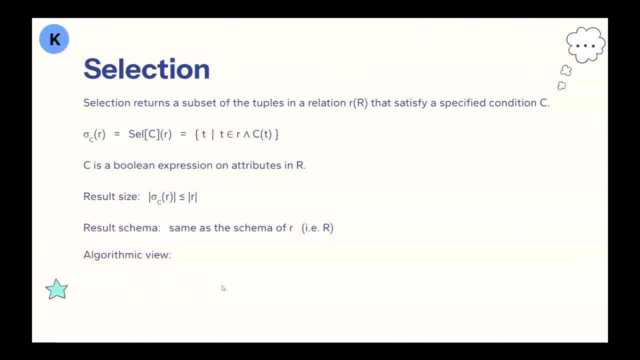 So that's the key, something you have to take note of, And here is an algorithm for doing this selection. So, basically, what we can do is we can just go through all the tuples in the relation and, if it fulfills the condition, 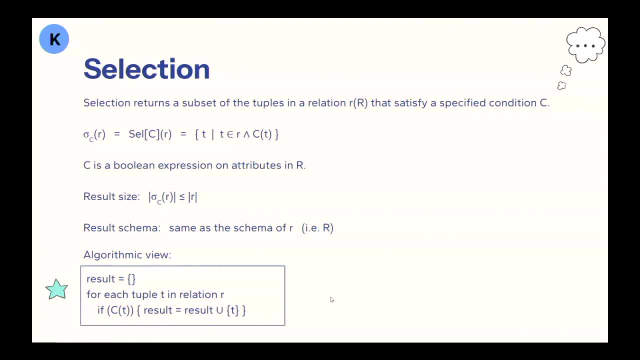 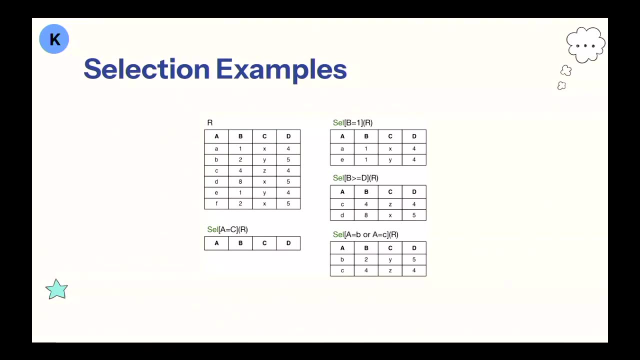 we will include it into the result. So that's the algorithm for doing selection And here's an example of. here are some examples for selection. So, as you can see, we can specify different conditions for doing selection And it will give us different results. of course, 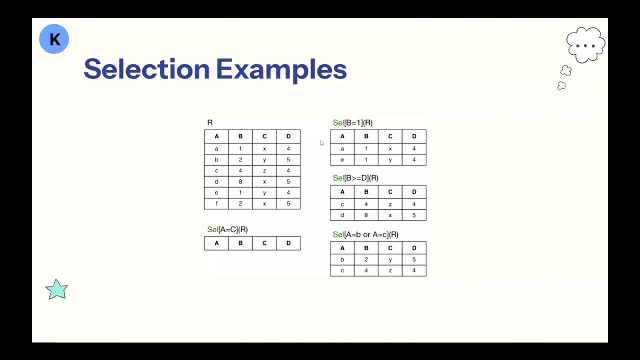 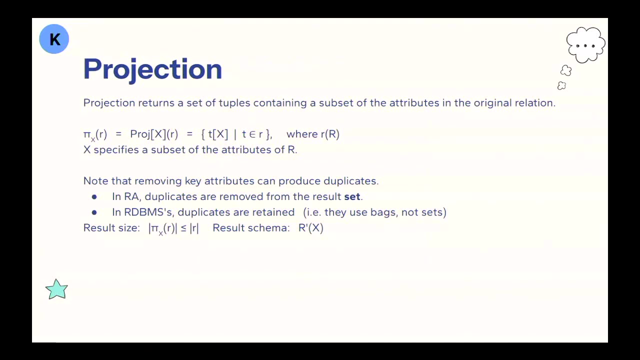 And another thing to take note of here is: the result will have all the attributes from R. So now you may wonder what if we just want to select a few attributes or a subset of attributes from R? what can we do? So we need another operation here, which is called projection. 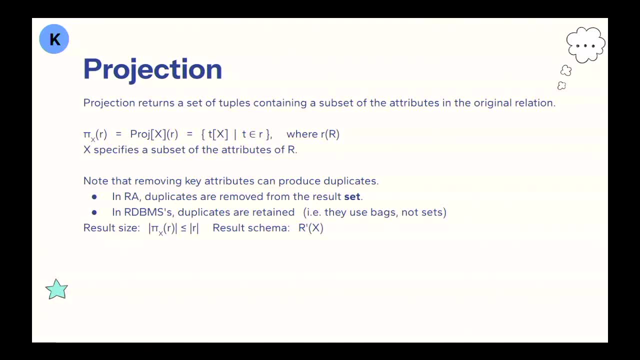 So production is used to return a set of tuples containing a subset of attributes in the original relation relation. so, as you can see, here, projection is returning a subset of attributes of the original relation. so so here you may. a key thing you you have to take note of is that if we don't, if in the production we don't select the 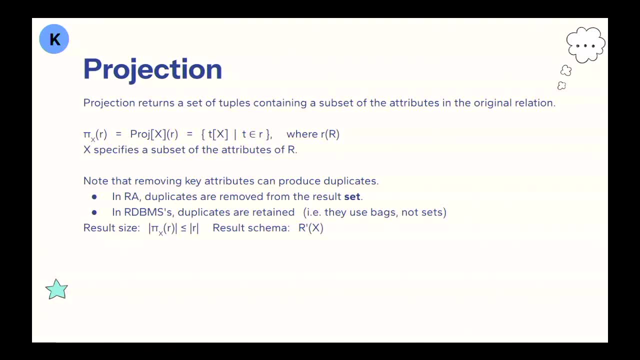 key, we may end up of having duplicates. and in SQL, if you don't select the key it, the result will include all the duplicate values. and because that's because for SQL queries by default, if you don't select distinct without, without a key, it it's generating a bag of values which allows duplicates. but 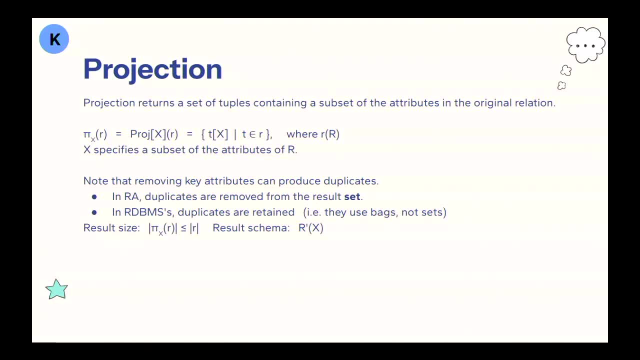 you, in relational algebra, duplicates are automatically removed because it's operating on sets. so this- this is a key difference between relational algebra and and SQL. and, of course, the result size is always smaller than, smaller than or equal to the number of attributes in the original relation. so 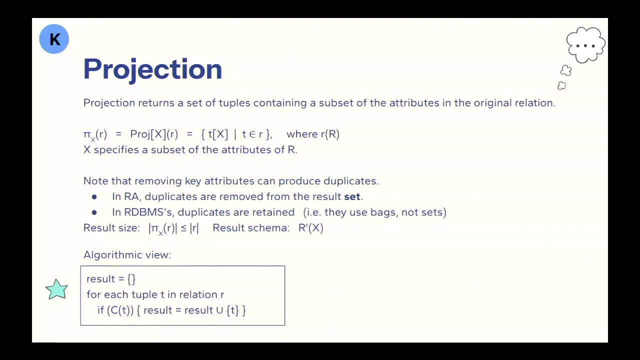 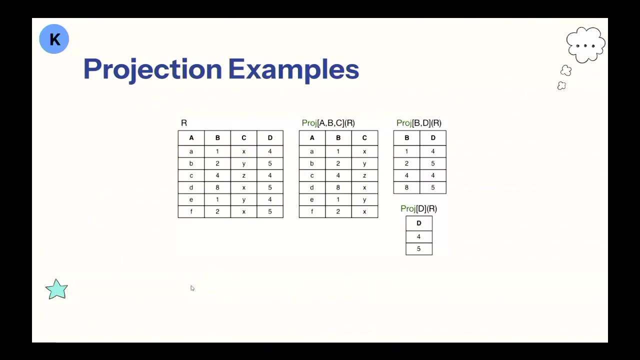 this is from the algorithm. this is the algorithm, so it's kind of similar to select, but instead of going through all the tuples, we are going through all the columns. so here are some examples for projection. so, as you can see, we can use projection to select entire columns and with the combination of projection and 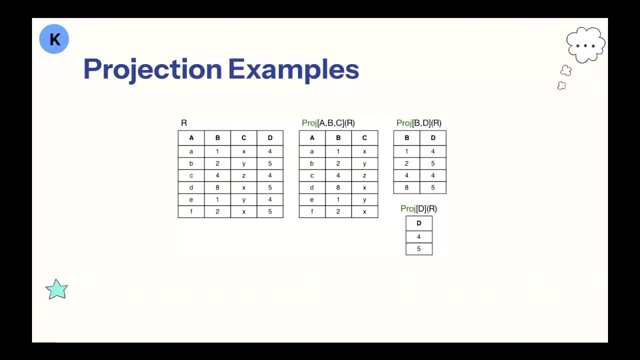 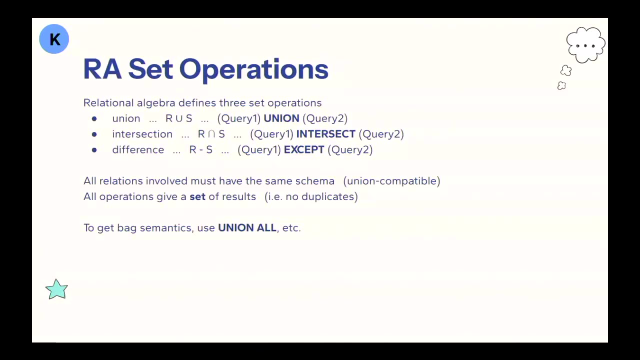 selection. we can somehow construct the select queries in SQL. as you can see, we can specify the tuple and we can specify the attributes. and now let's? now we have learned how to, how to extract certain, a particular value from a given table, and by locating it the the exact column and row. and now let's learn some set. 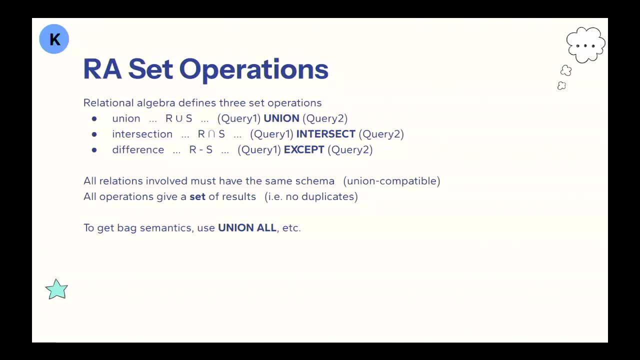 operators for us to manipulate the results or the relations. so relational algebra defines three different set operators. the first one is called union, so union. the concept of union is very similar to the concept of a, two, two, two to the mathematical concepts in the set theory, and intersection is also the same. 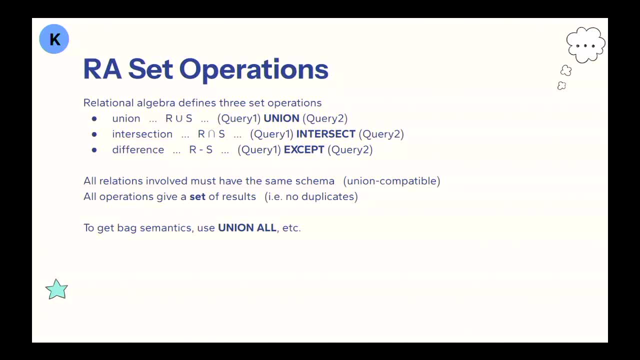 and another thing here is called difference. so it's also very similar to the set operators of what we have learned in SQL. so for union and intersection the order doesn't matter. so our union s and s union R will give us the same result. R intersect s or s intersect R will give us the same. 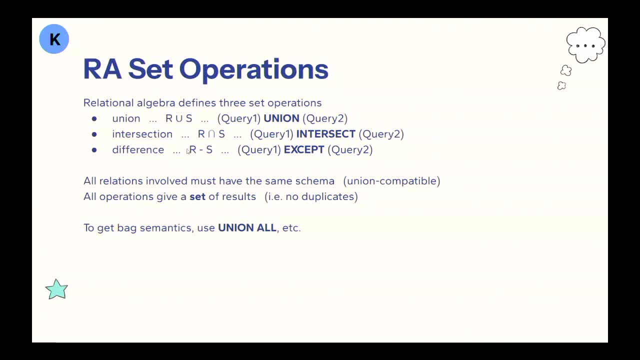 result, however, R minus s and s minus R will give us different results most of the times. so all here. for in order to use set operations, all the relations in both as operands must have the same schema, so in other words, they must be union compatible. so that's the first requirement here, and the second 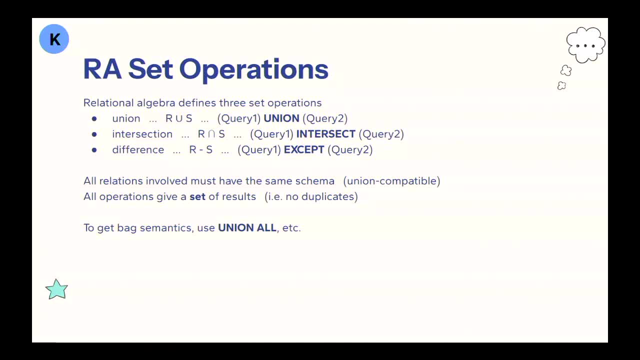 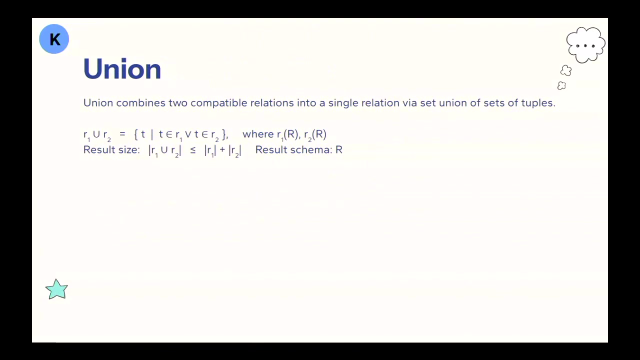 restriction here is: all the operations will give us a set of results and the behavior is quite similar to SQL. so in order to, in order to get back, we need to word all. So this is: here are the set operators. So for union, the concept is kind of straightforward. 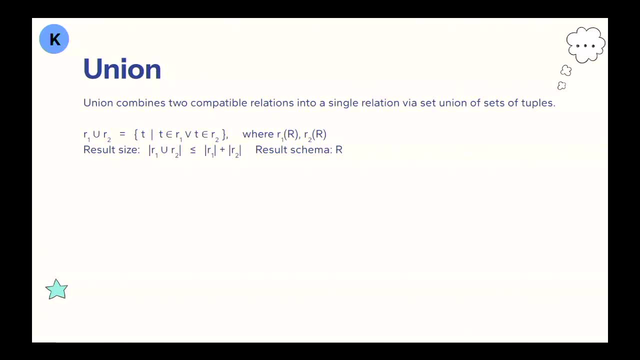 It is used to combine two compatible relations into a single relation. We are set union And in this union step all the duplicates are removed And the result size is always smaller than or equal to the combination or the combination of the size of the individual. 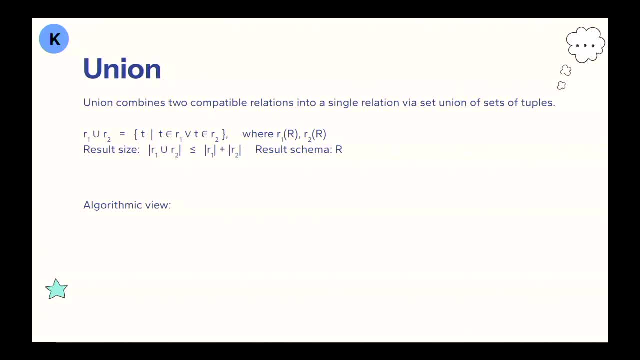 relations. So if there is no duplicate, the size of the individual relations is the same. The size equals to the size of R1 plus the size of R2.. If there are duplicates, the size of the result relation is smaller than R1, size of R1 plus size of R2.. And here is the 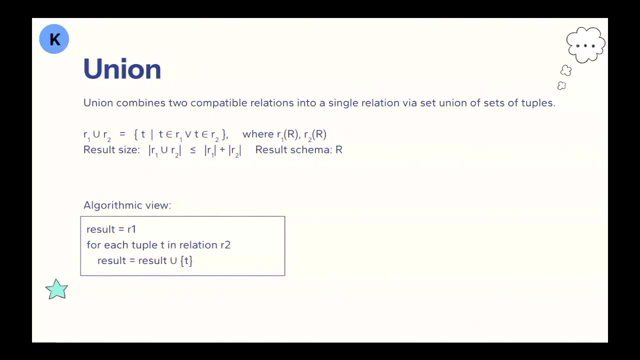 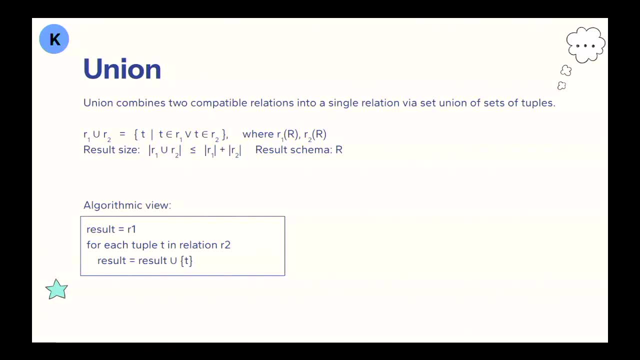 we introduce the items of the second, the second relation, one by one. So there's the, the algorithm here, And the concept of intersection is is defined as it is to combine two compatible relations into R2 and R3. relations into a single relation where the set intersection of sets of tuples. 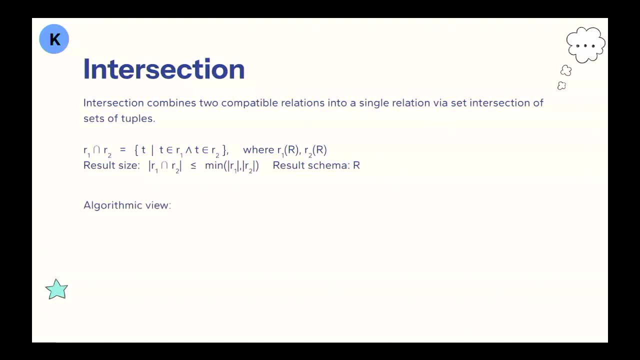 So the concept is very straightforward as well, And the algorithm here is: we initiate the result set as an empty site, And, for each tuple in one of the operands, we check if this tuple appears in the other operand And if so, we will put it into the result. 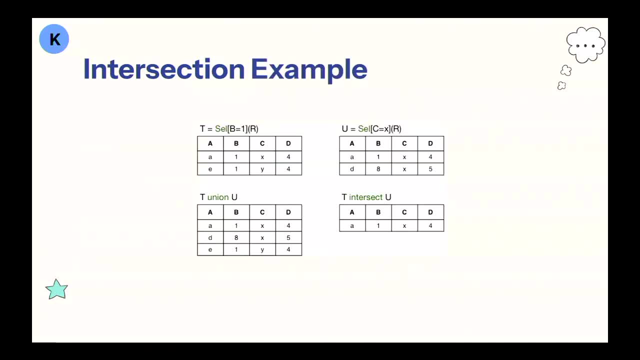 So that's how we do intersection And here are some examples for unions and intersections. So, for example, for t, we have this, For u, we have this. The union is To combine, To combine them together and remove duplicates. 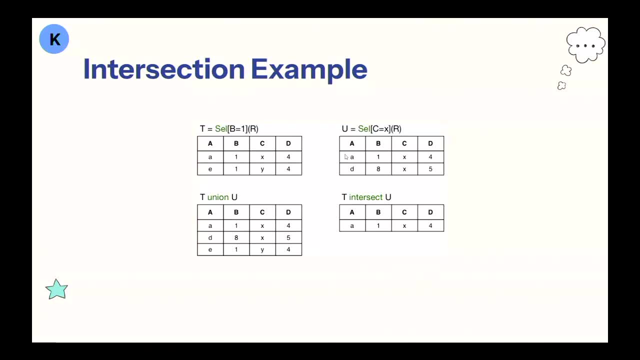 For the first row they are. they are essentially the same. So only only one instance of the first row appears in the result And, as you can see, here the restriction is the two. the two operands must have the same schema here. 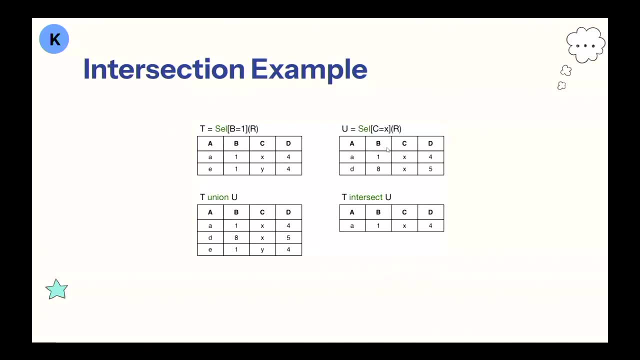 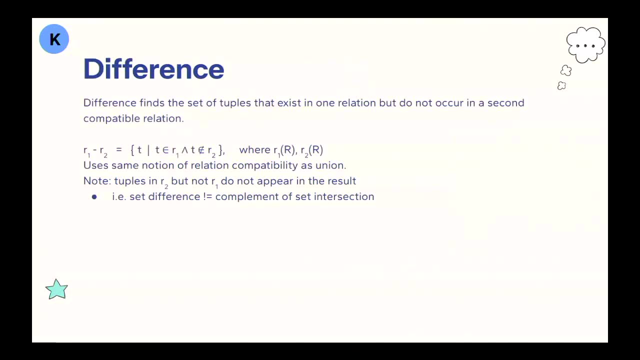 So they must all have a, b, c and d as their attributes. So here here's the example. And the last operation, the last operator for sites is called difference. Difference is used to find a set of attributes that exist in one relation. 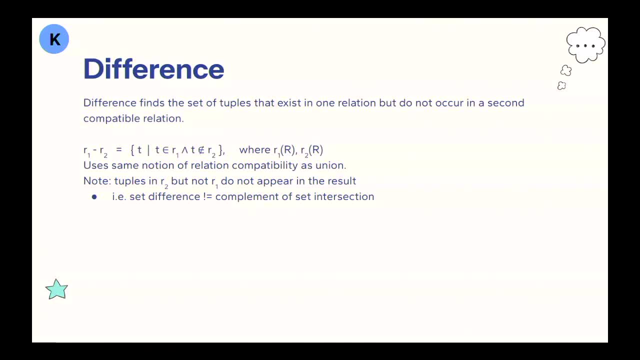 But do not occur in the second compatible relation. So it's it still requires the the two relations to to be compatible, To be union compatible, Which means that they must, the two operators, the two operators must have the same set of attributes. 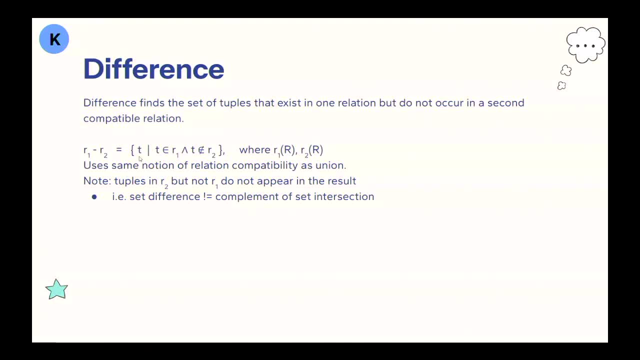 And and, as you can see, the condition, the set condition here is essentially reflecting the, the fact that a tuple must appear in one of the in the left operand of the set And it shouldn't appear in the right operand. 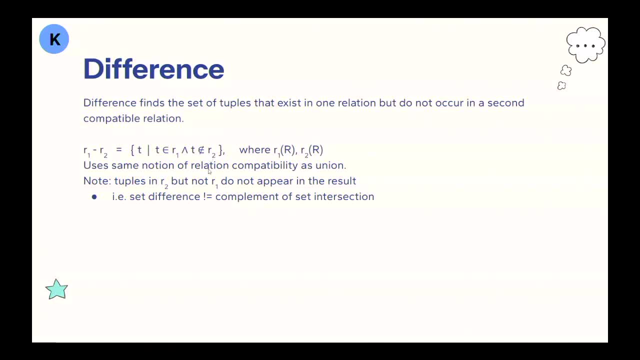 So the, the, the outer matters here. And from the mechanic, from the mechanism, it is actually like the complement of site intersection, It's like removing the intersect or removing the intersection from the left operand. So this is the, the operation of difference. 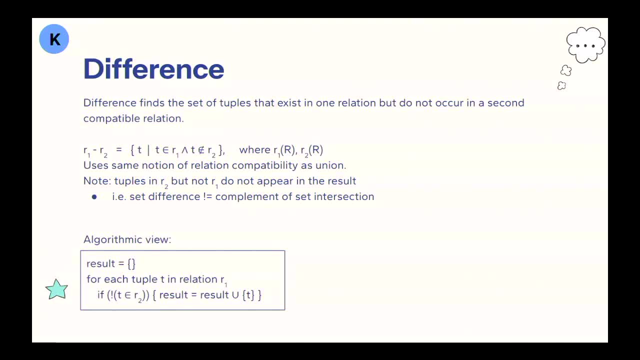 So the algorithm. from the algorithm point of view, this is how we can implement site difference. As you can see here we just need to change the. we just need to reverse the condition here from how we calculate intersect. So we just, instead of t from r, t, t is in r, r2.. 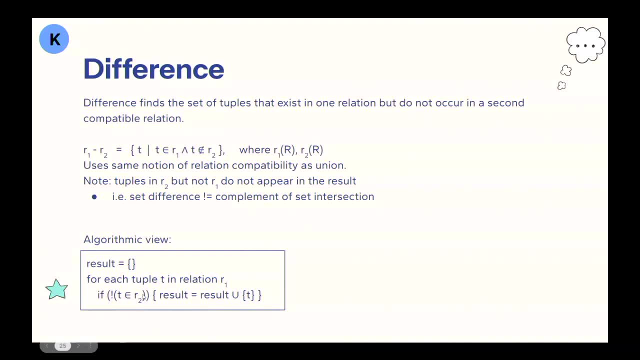 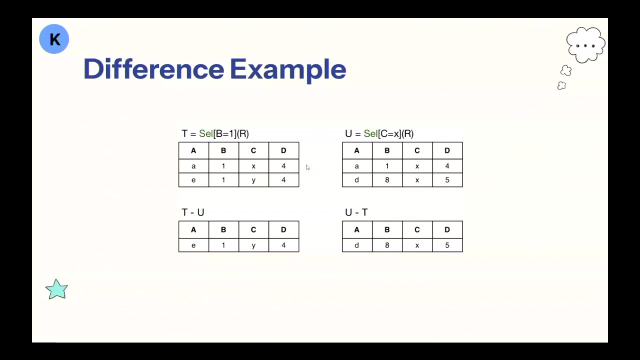 We should use. t is not in r2 here. So that's why difference could be considered as the complement of site intersection. So here is an example of difference. So you do notice that the outer matters here. So you have two key things to take note of here. 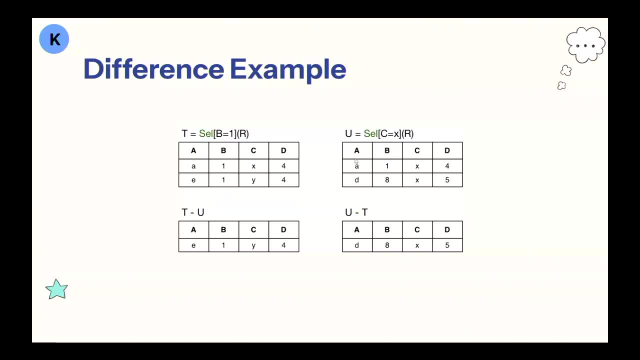 The first one is they must be union compatible, which means that they should they should be union compatible, They should have the same set of attributes for the two operands. The second thing here is the other matters here, So only the only the, the. 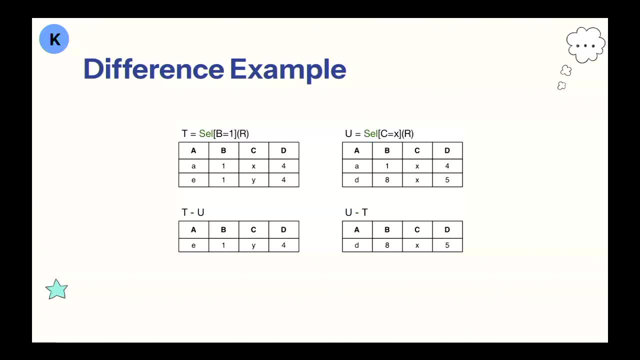 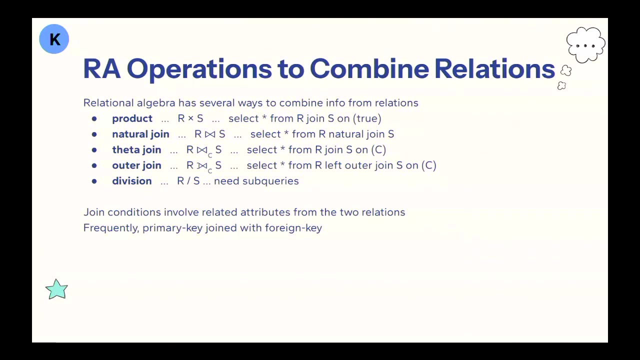 the result, or the tuples in the right- left operator is kept in the result. So this is the, an example of difference And we can and. and another thing after covering the how we select the data Using selection and projection, And after learning how to combine results using set operators. 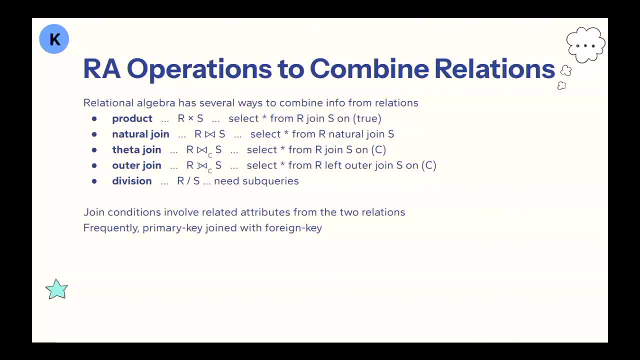 What we are going to. what we are going to learn is: how can we combine different tables Or combine different relations, And relational algebra has several ways for combining these relations, And is it? it has a mapping to the join operator of SQL queries. 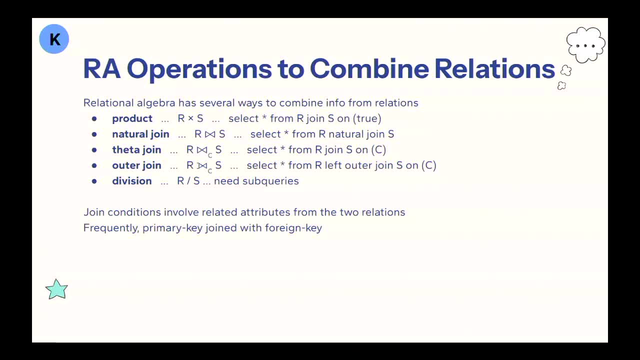 But the but, some of them, they don't have an exact match. So the first, the first concept here, or the first operation here, is called product. It is, it is the Cartesian, Cartesian product. So it will give us a very large table in this. in this sense, 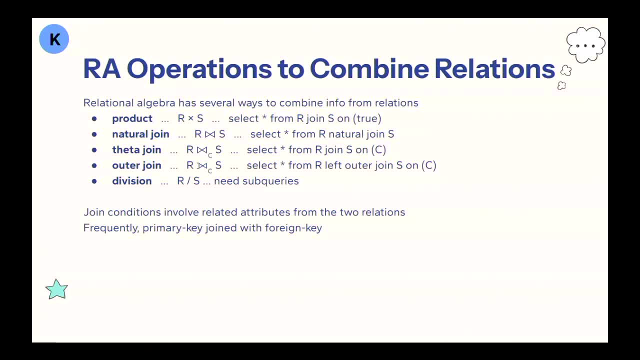 We will learn that later. And the second concept here, the second operation here, is called natural join. So it is to join two tables on the common attributes. The third one is theta join. It is to join two tables that fulfills certain conditions. 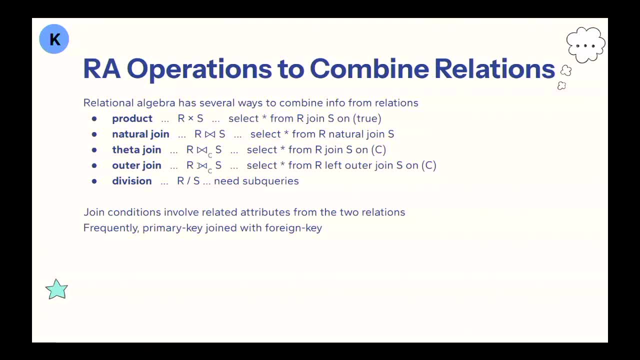 And the fourth operation here is called outer join. So, as in this example here it is a left outer join. You can see there are two small extensions here in this symbol, So this means it's left outer join. So Well, The concepts of these. 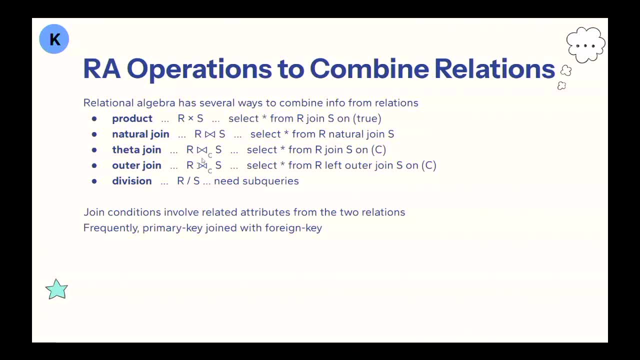 These three joins are kind of similar to to what we have learned in SQL. And the last, the last operation here is called division. So in division there's no single query that in SQL that could do this division. So we need some sub queries to do to do it. 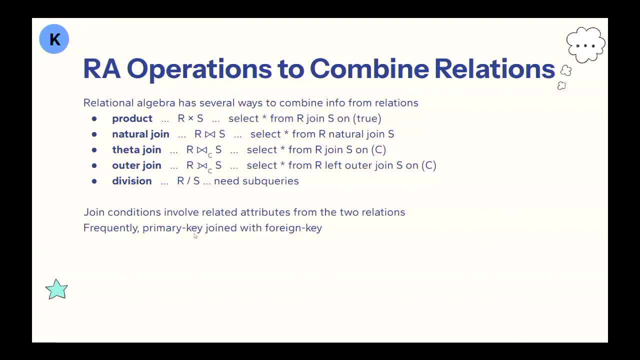 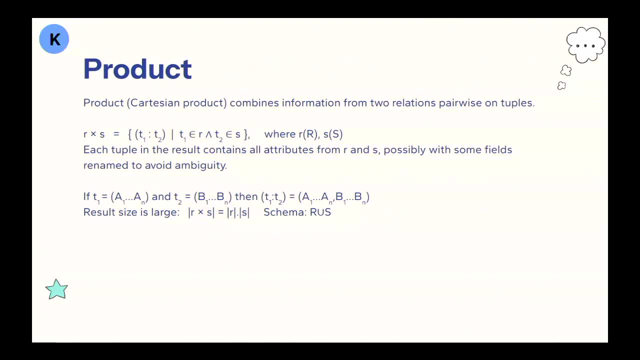 And we will learn this later. So first let's learn product, or Cartesian product. So it it is to combine information from two relations, pairwise on tuples. So so it is like it will result. it it will give us a big table. 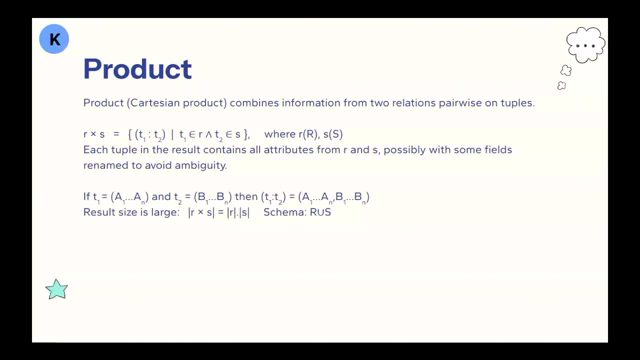 Combines every permutation. So So It itinstall Of the combination of tuples in the first table and tuples in the second table. So it is essentially a product. So the, the, the size of the, the size of the. 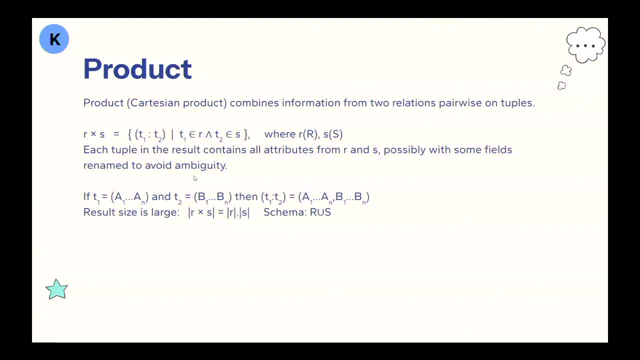 the result is the size of equals to the size of the size of the first, the first relation times The size Of the third relation Times size of the second relation. so this is the, and the schema will be a union of. 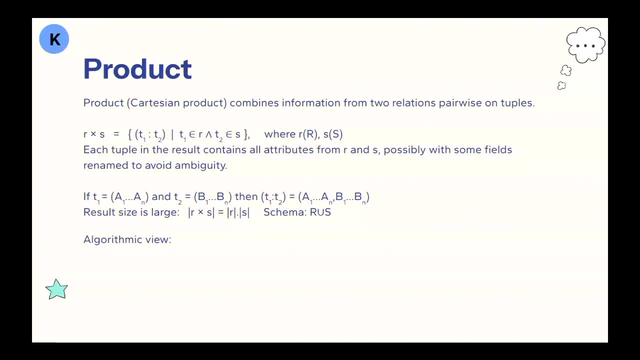 the attributes from the two operands and this is the algorithm of calculating product. so essentially we will have two loops. so first we will go through all the all, the all the tuples in the first operand and then we attach, and for that tuple we build a pair with every other, with area tuples in the second table. so 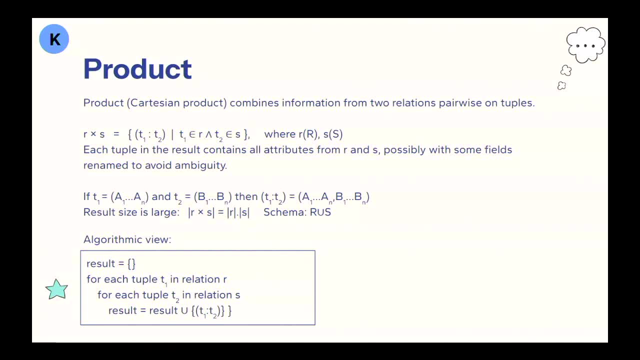 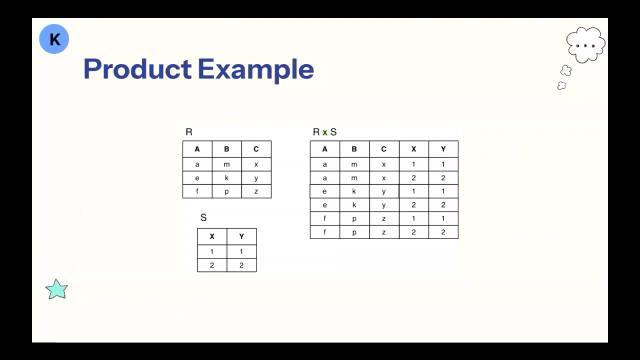 so this is how we do product. it will give us a very, very big table. so this is the example here. so, for example, if we want to, we want to get the result of the product of R and S, what we will do is we for, for each tuple of R, we create for each tuple of R. 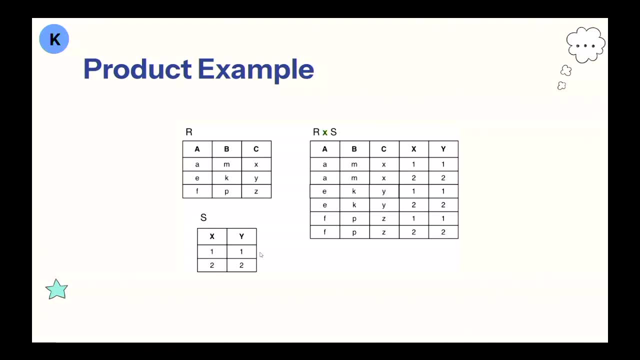 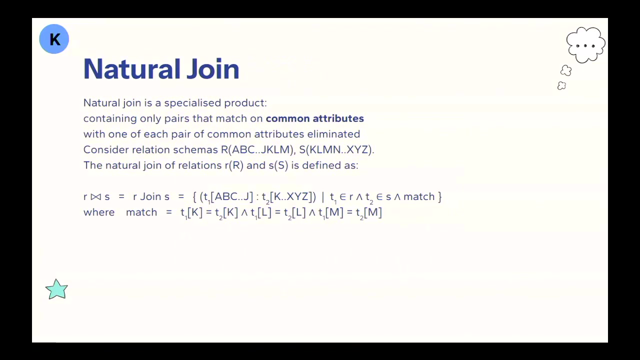 we create a set of tuples for for each tuple of S, so we combine it with each tuple of S to create the product form, a new tuple. So that's why the size of the result equals to the size of R times size of S. So this is called product. And the second operation here is: 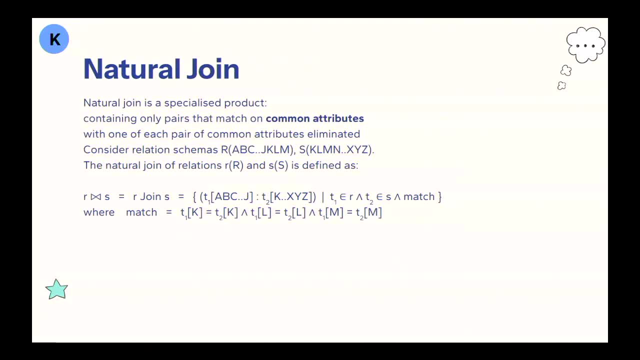 natural drawing. So natural drawing is a specialized product, So we don't specify. we don't specify a condition here. We don't specify a condition here. However, since it is natural drawing, we are drawing two tables, naturally And in order to draw. 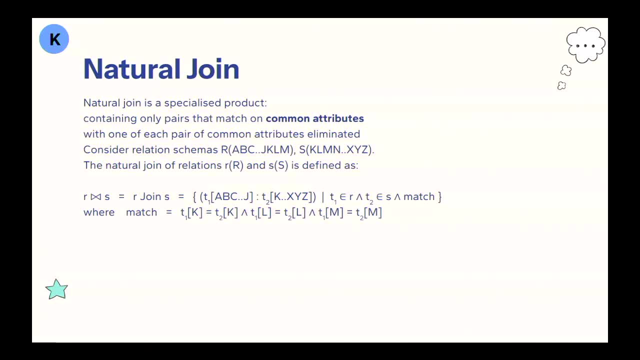 them. naturally, we need to find out the common attributes And we draw in the tables on the condition where the common attributes of table R equals to table S. So this is how we do natural drawing. So from the algorithm point of view, we are adding a condition here. We are adding a condition. 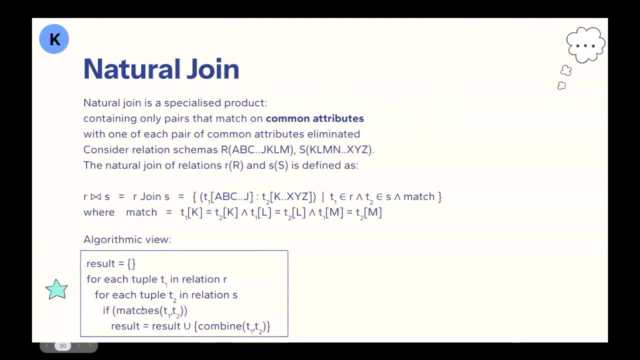 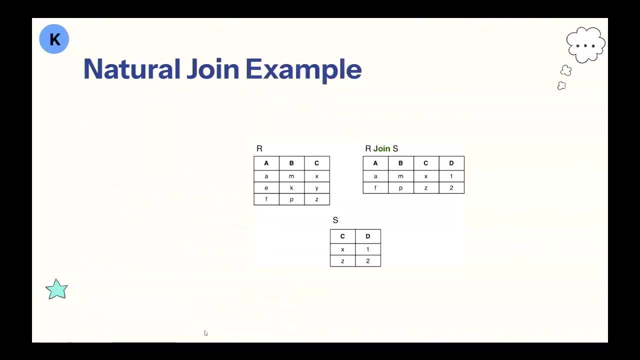 here when we loop through the tuples of each individual operand. So if the attribute matches with table R, we will combine them together, otherwise we don't. So this is an example of natural drawing. So for R we have attributes a, b and c For 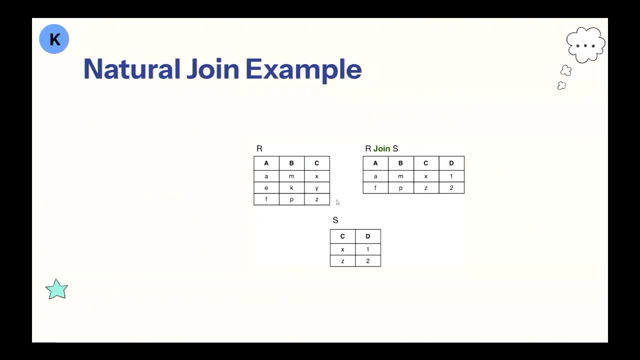 S. we have the attributes of c and d. So when we do natural drawing we are drawing these two tables according to the value of c, So only if the, the value of c, matches the value, we join the tuples together. so that's why in the end we will have a table of 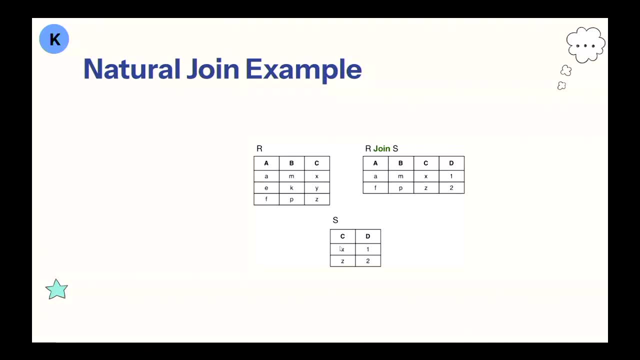 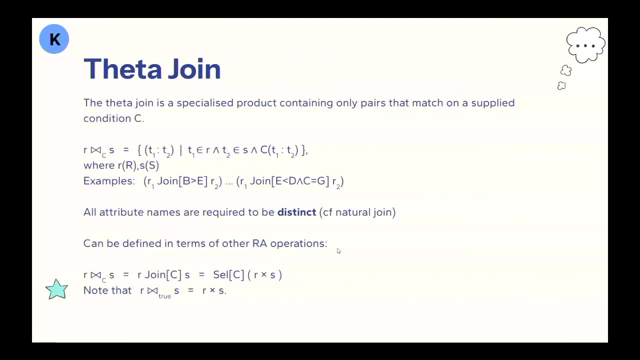 two tuples because because of the unique values of C here provided by S and theta join. so actually all the other joins are specialized product, so is they are all created by adding conditions for the Cartesian product. so the theta join is a specialized product containing only pairs. that matches on a supplied. 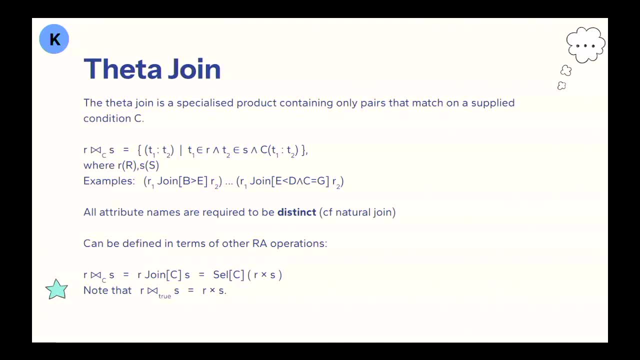 condition here, so you can view it as a generalized natural join. but but the difference here is that all the attribute names requires to be distinct. so for natural join you need to be distinct. so for natural join you need to be fair. to join the the toward tables should have, should have, should have. 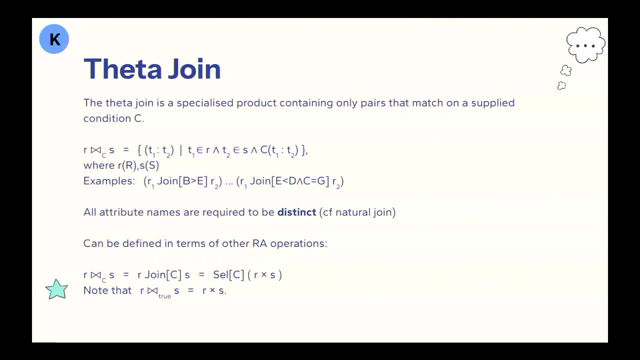 common attributes. but for thickness wine they don't. they don't, they shouldn't have common attributes. so our names should be unique. but we can specify the condition of joining here. so instead of panning ira top hole with in one table with Airy top hole from another table, we can't add some conditions to filter? 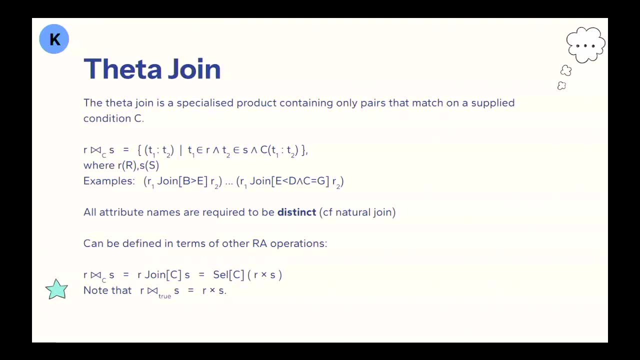 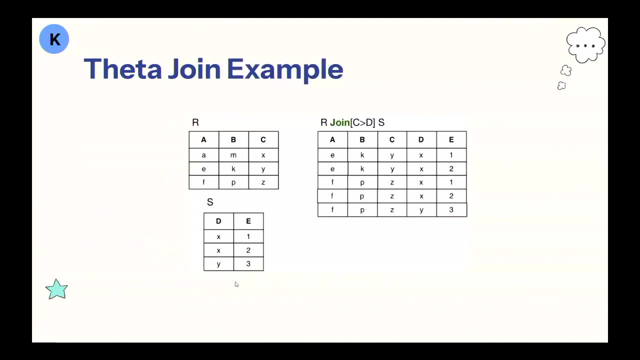 out some of the permutations or pairs here. So this is the concept of theta join And this is an example of theta join. So, as you can see here the two operands should have different set of attributes And we can specify the condition here for joining the two tables. 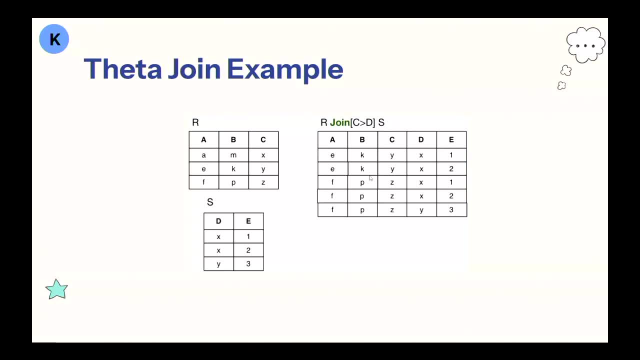 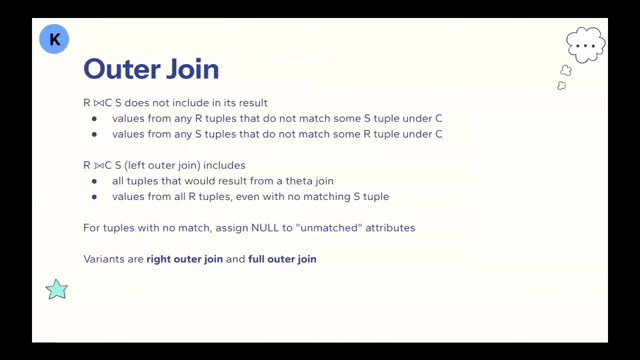 to filter out some of the pairs. So this is how we do: theta join And the last join here is called outer join. But this is not the last operator here, So last join is called outer join, So outer join. so for natural join and for 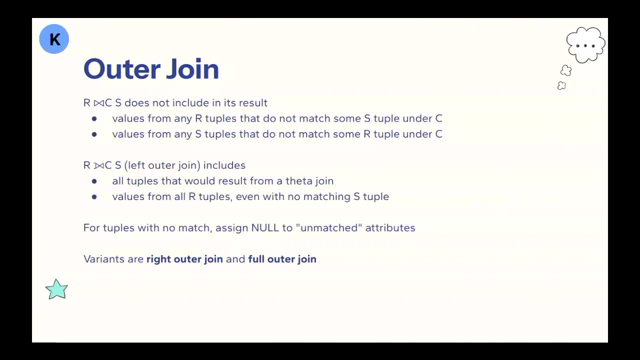 natural join. what we do is we don't include values from any operand, the tuples from any operands, that there's no matching. There's no matching from the other table, from the other relation. So this is the theta join and natural join. 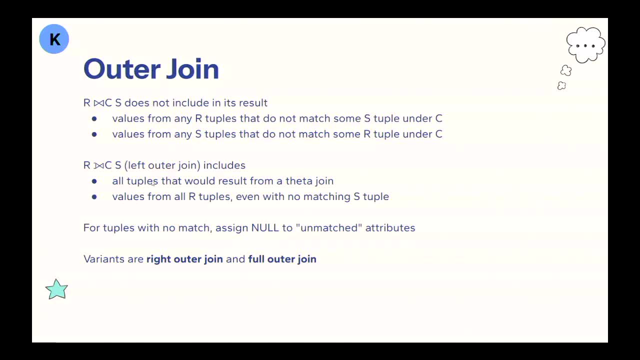 But for outer join Other than the other than the tuples or pairs of tuples fulfilling the conditions, we also include the tuples from a particular operand relation. So for left outer join we are including all the all the tuples from the left operand. 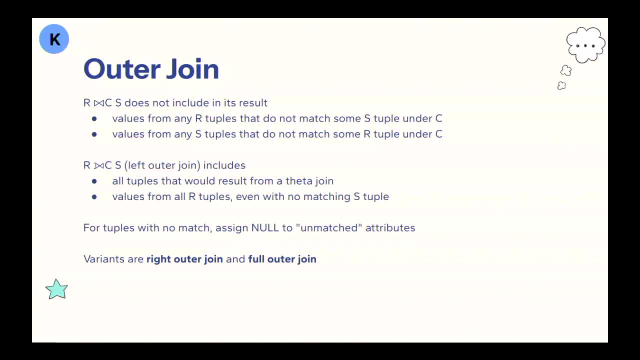 For d right outer join, we are including all the topos from a particular operand, the tuples from the right upper-end, And for full outer drawing, we are including the tuples from all the two upper-end relations. So this is actually very similar to what we have learned in SQL. 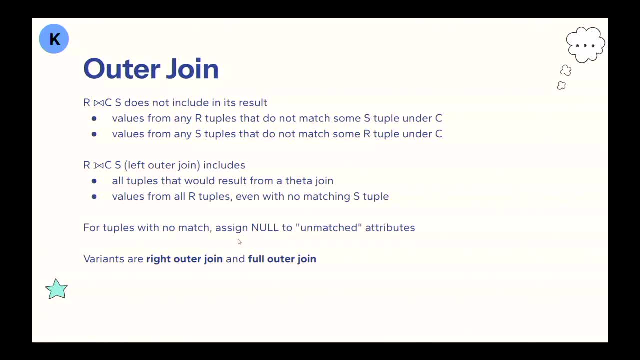 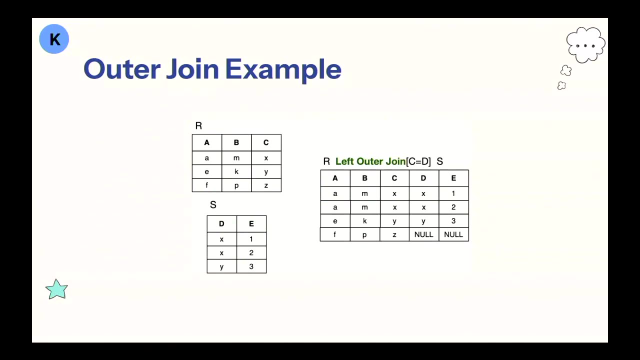 And the default behavior is also similar. So for unmatched attributes we are assigning the default value of now. So here is an example of left outer drawing. As you can see, here for the A value equals to F. there's no, actually for this third row of R. 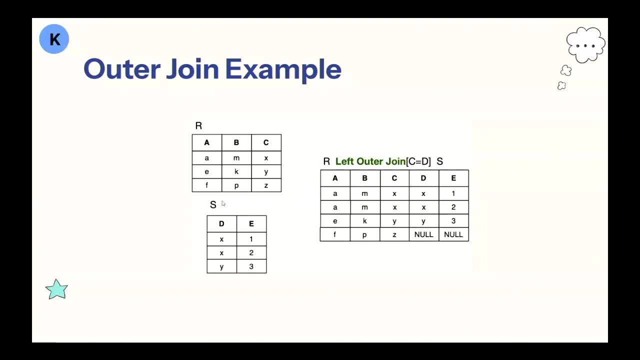 there's no matching in the table of S. So, because C equals to Z in this case and there's no D equals to Z in the table of S, so there's no matching for this row here and we will put the default. 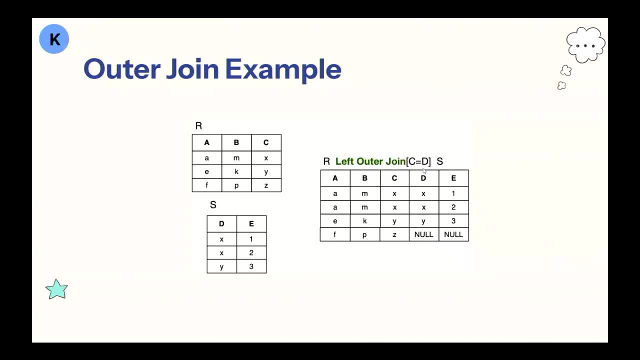 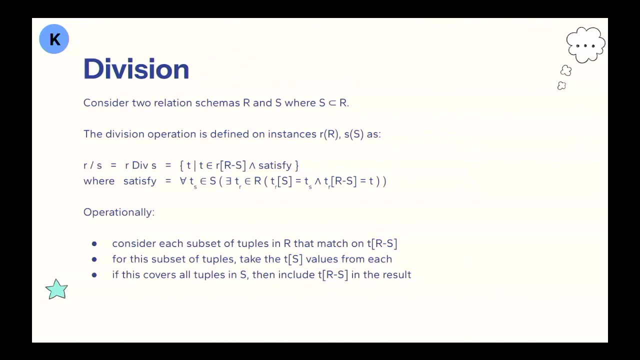 we have still included into the end result, but we will set the values of D and E to be now. So this is the mechanism of left outer drawing, And those drawings are very, very similar to what we have learned in SQL And there are small differences, but they are essentially very similar. 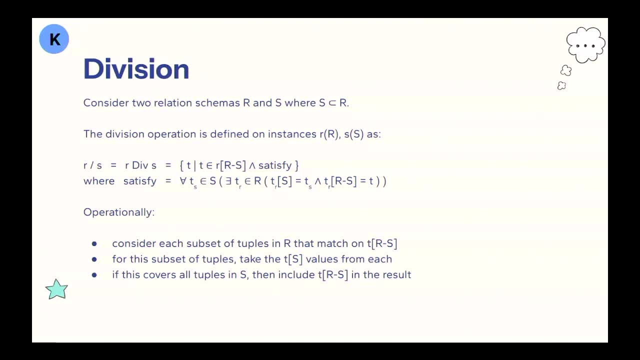 And the new concept here is called division. So for division there's a restriction of the two operands, So one of the operands must be a subset of the other one, So the right hand side operand must be a subset of the left operand. 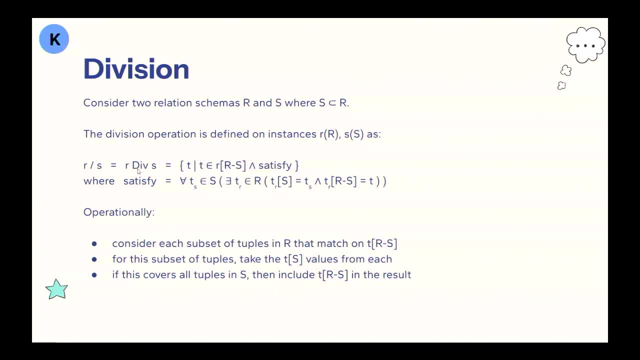 And R divided by S is denoted as a set of tuples, T, where T has the attributes of the attributes R, minus attributes of S. So the difference of R and S will go to the tuples of R and S. So the difference of R and S will go to the tuples of R and S. 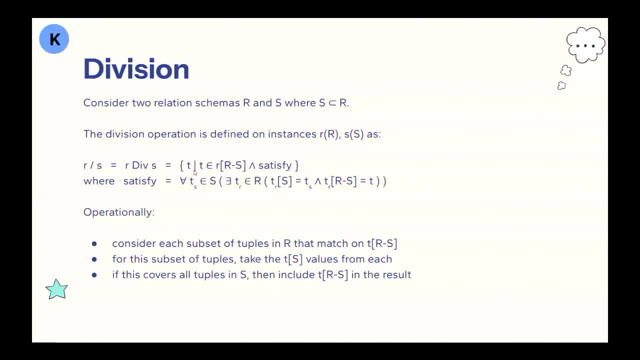 So the difference of R and S will go to the tuples of R and S. So the difference of R and S must have an appearance or occurrence in the table of R in the left operand. We will show you an example later, but don't get worried about the concept here. 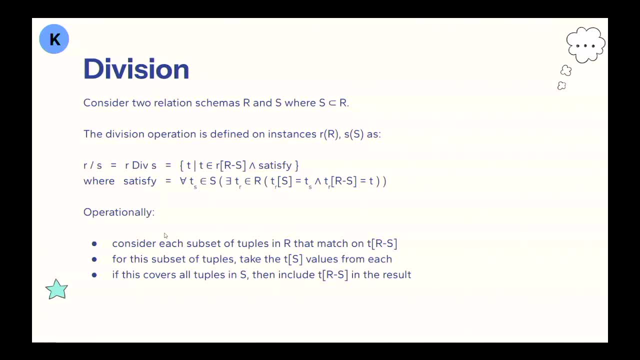 So operationally how we collect the division here is like: consider each subset of tuples in the left operand. We will show you an example later, but don't get worried about the concept here. So operationally how we collect the division here is like: consider each subset of tuples in the left operand. 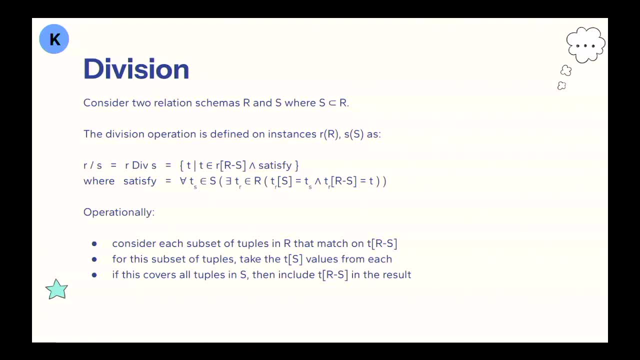 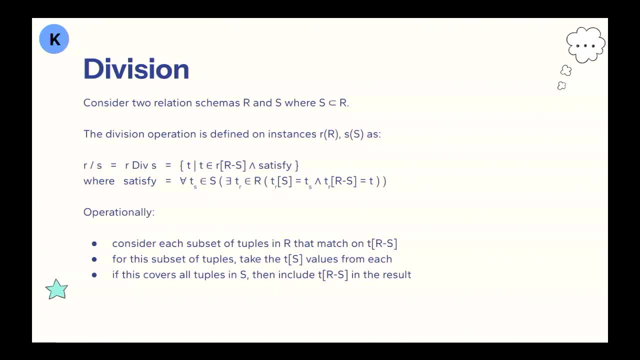 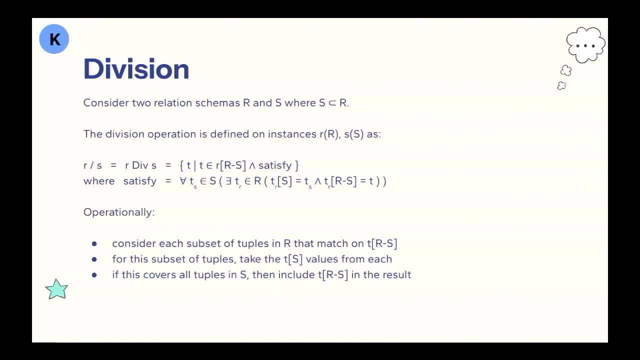 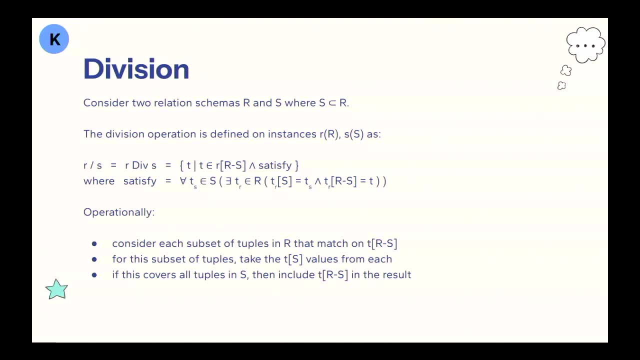 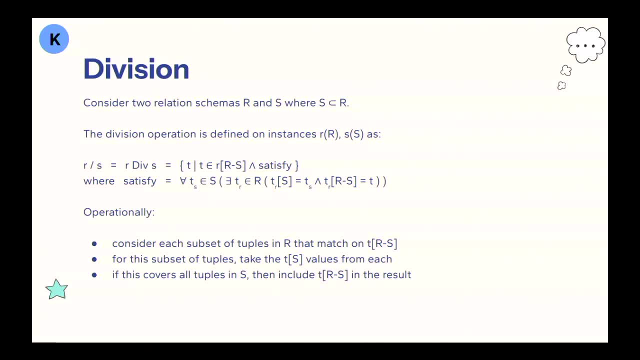 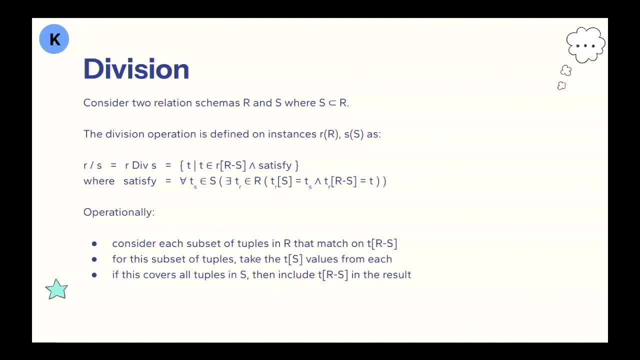 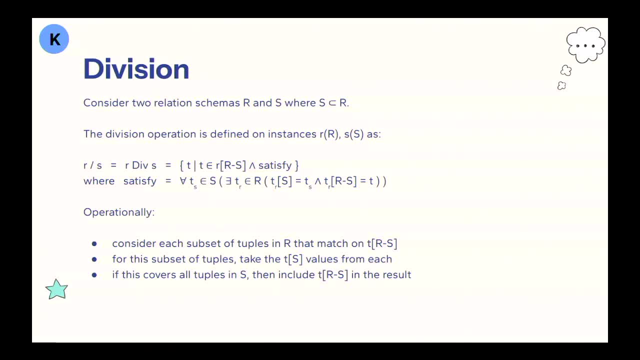 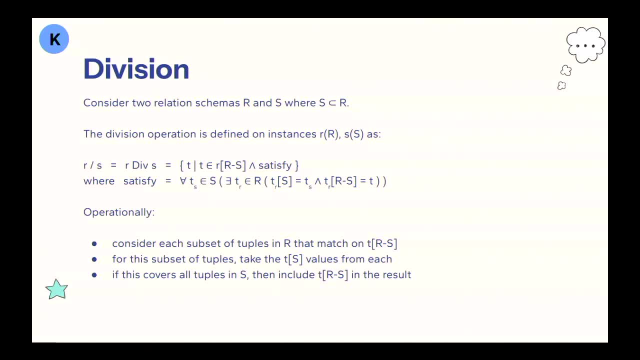 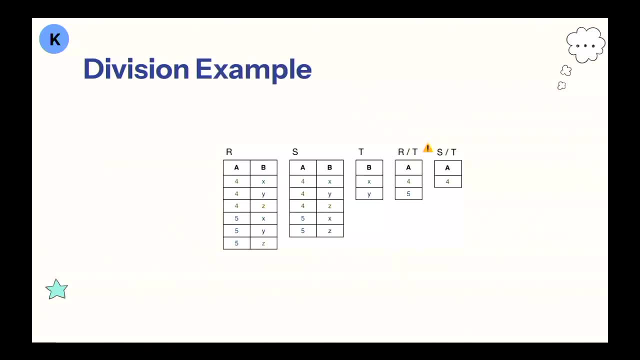 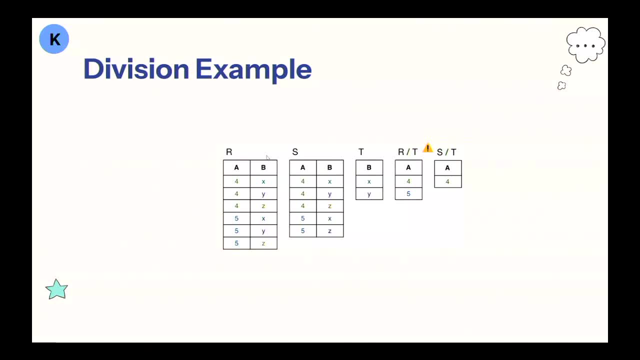 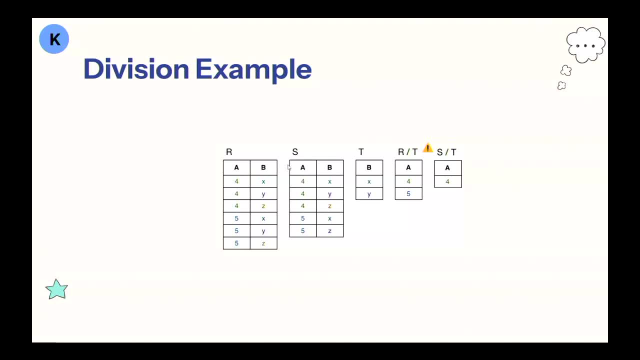 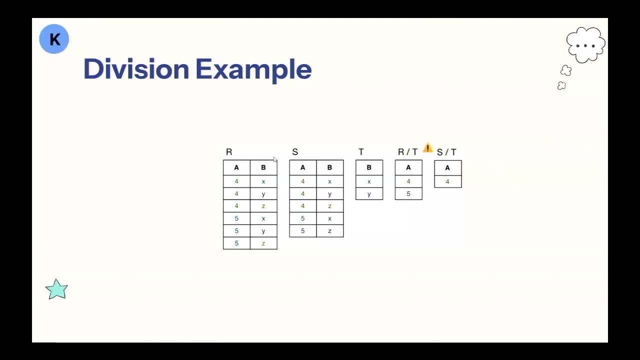 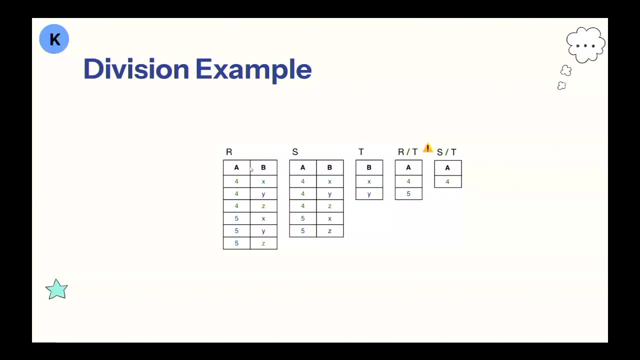 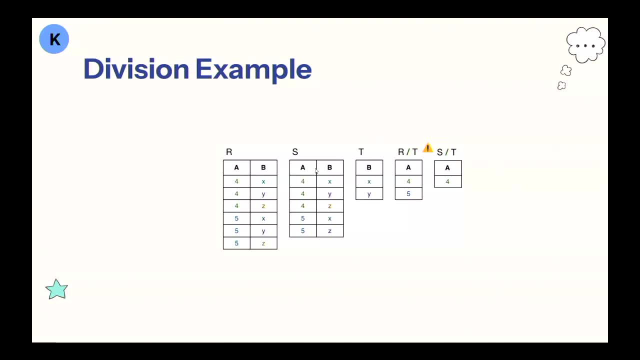 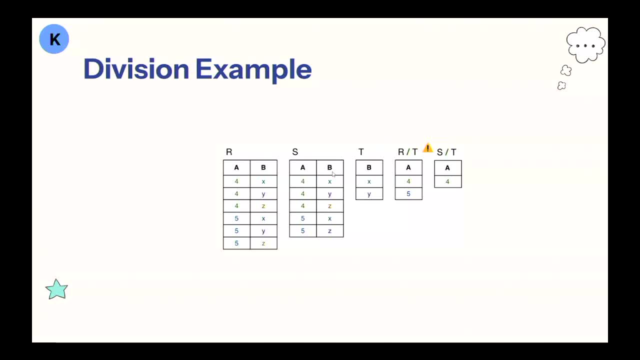 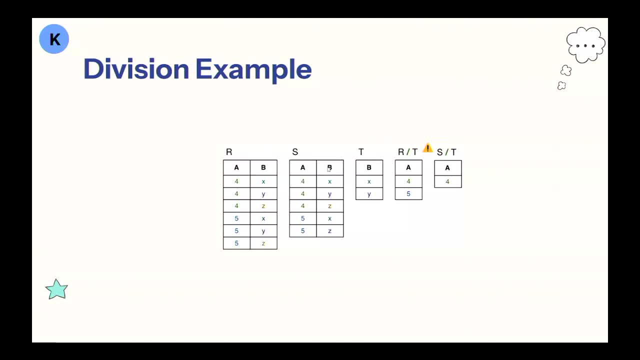 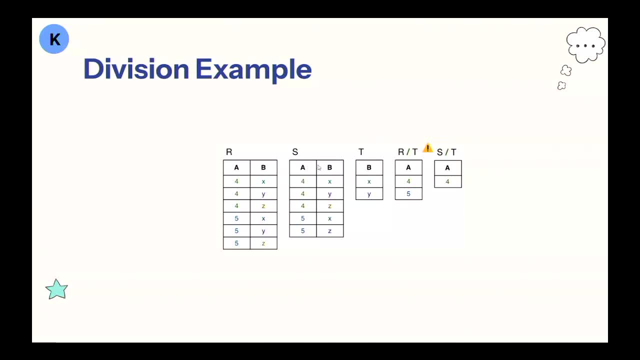 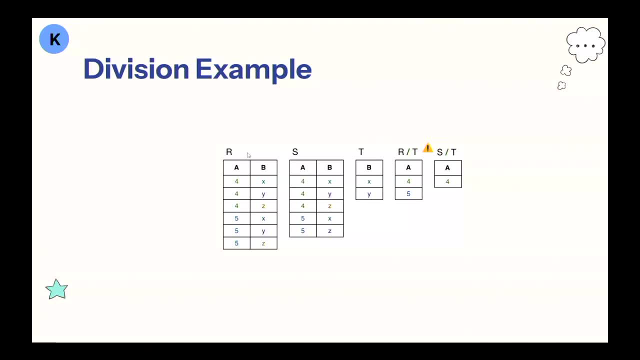 And for this subset of tuples we take the value from the table of the right operand by R or S, Because we can't divide. it is like we can divide a larger table with a smaller table, but we can't divide a smaller table by a larger table. And here is the result. 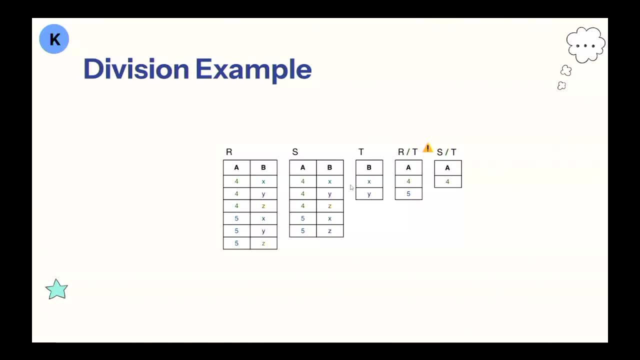 of R divided by T, So for T. this is how we do it, So the result should include R minus T, the attributes of R minus T. So what is the attributes of R minus T here? So the difference here is A right, So the result should contain attribute A here. 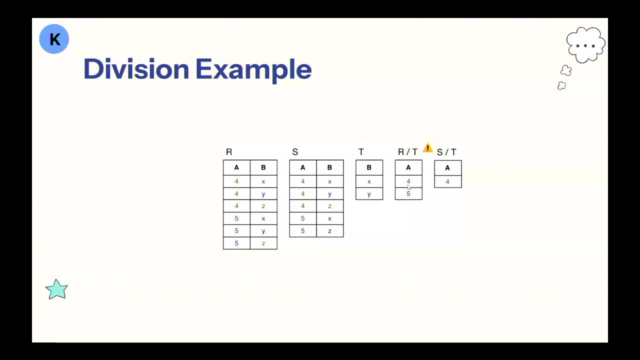 And how can we get the values here? So now we know. okay, the result should have attribute A. but what about the values? The values is like this: For R divided by T, we can see that for because T has X and Y. for the value of B, And let's go through the column or the 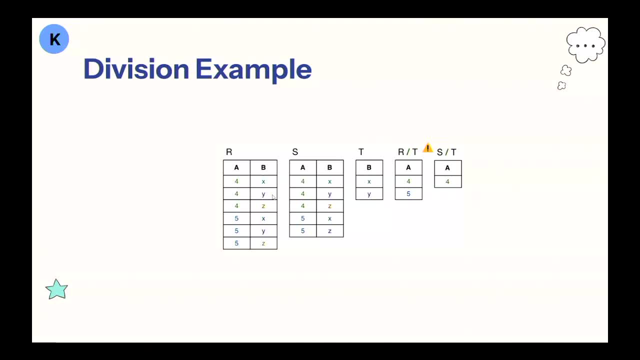 attribute values of B. Here A will be basically the eight times the recurs Tor, so theörper Y is the number of terms. X and Y is in R times 4.. But X and Y is equal to 4 or above. What is the し? 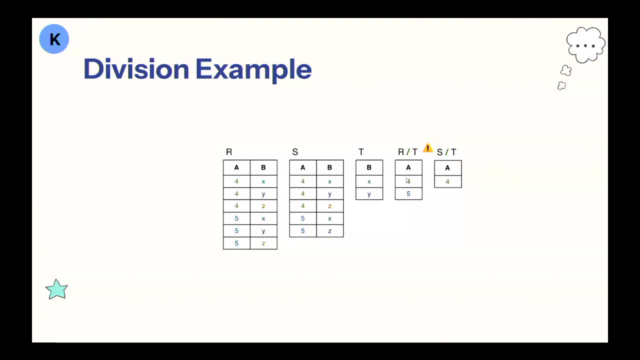 recover Why y lives in table R. Well, we know that instead of y moving from table A, x is going to move to table A. So what does the Vale to be equal to in table R? so we should put the value 5 of A in the result. This is how we 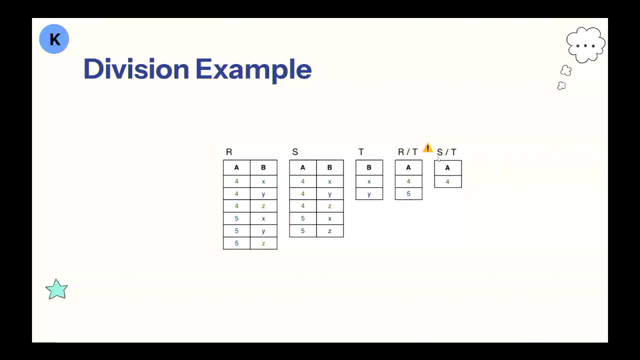 calculate R divided by T And for S divided by T, what we are thinking. the thinking process is kind of similar. So first let's determine what which attribute should be put into the result. So the result should be S minus T. 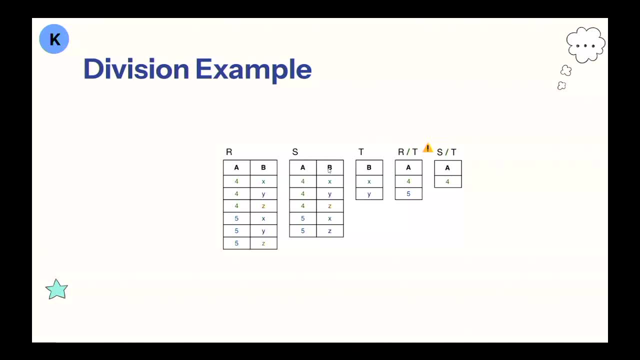 And S minus T is is actually the same as R minus T is A. So we should put the attribute A into the result. And to determine the values, let's go through the table: the values of B in relation S. So remember, for T the value of B could take X and Y And and in this table here 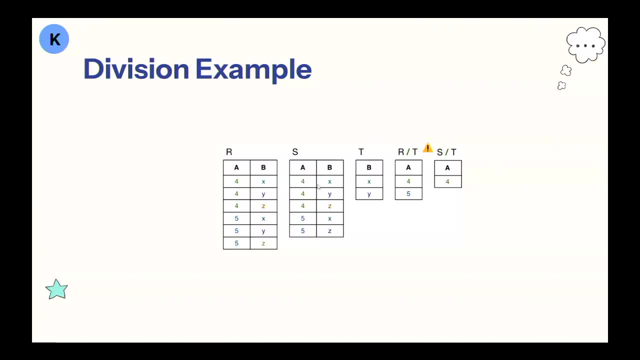 when A equals to 4, B can take both X and Y, so that's why we should put 4 into our result. However, when A is equal to 5, The value of b can take x or z. It doesn't cover all the values of t. 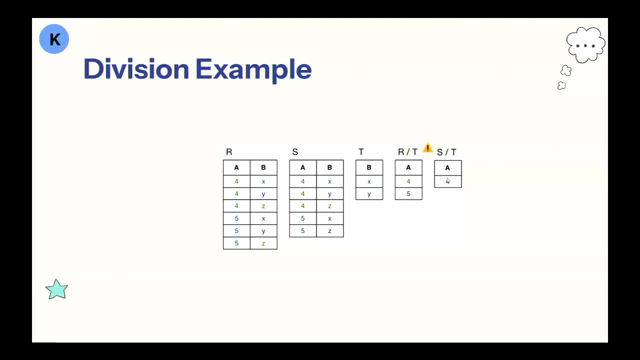 So we shouldn't include 5 into the result. So this is the definition of division. So it is like how you do a numeric division. So it is like the divisor here must have its entirety, The entire appearance or occurrence in the divided value. 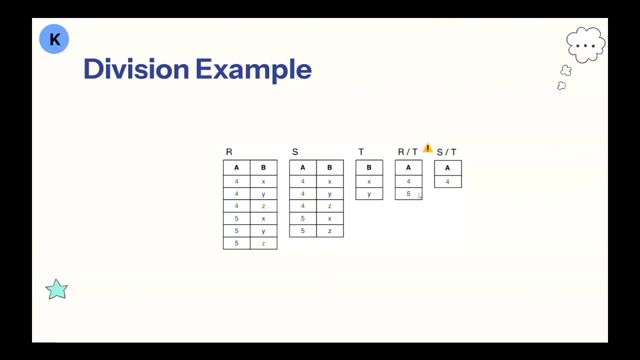 So that's why we should. that's how it works And that's why there's a difference between r divided by t and s divided by t. So this is the concept of division, And let's have a ten minute break before we come to the 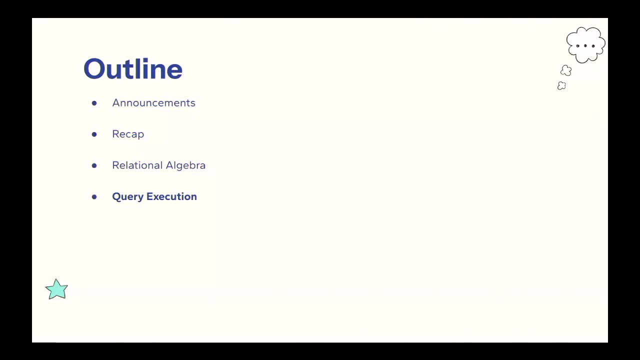 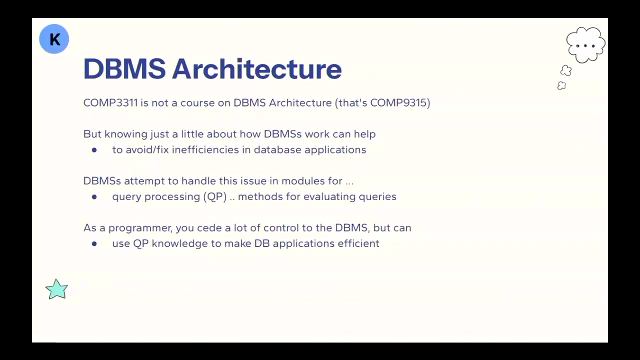 all the relational algebra. so you may wonder: okay, why are we learning these concepts? it's because they are actually very, very useful for for dbms to do optimizations, or they are actually the, the so-called machine code executed by the dbms engine. so let's learn. how does dbms 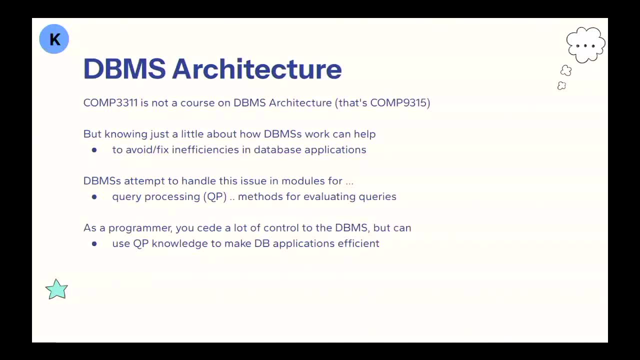 execute queries. so this, this course, is actually not a course on the active architecture of dbms and that course is actually a graduate course. but knowing a little bit about how dbms work can help can help you to avoid or fix the efficiency issues in your applications. so it is like if you know what 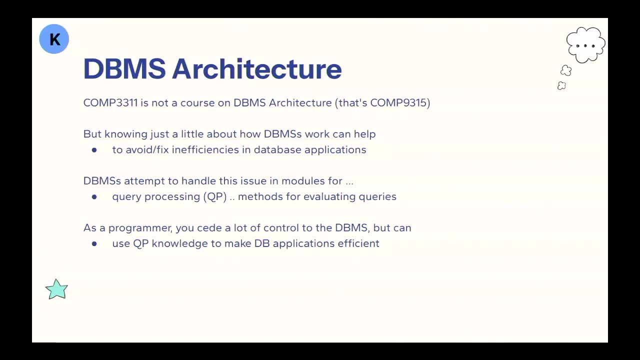 you're doing the mechanism of python or c, the python interpreter, or c compiler, when you write your program. you can optimize your program. so it's similar. if we know how the dbms works, how this engine works, we will, we can somehow optimize the queries we are writing. so 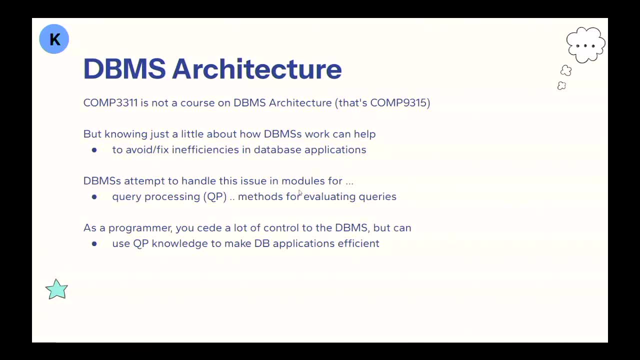 so dbms is trying to handle this efficiency issue of the user provided query with a module called query processing and it has several methods for evaluating queries and and you can use this knowledge to make your application more efficient. so this is our view of dbms so far so. 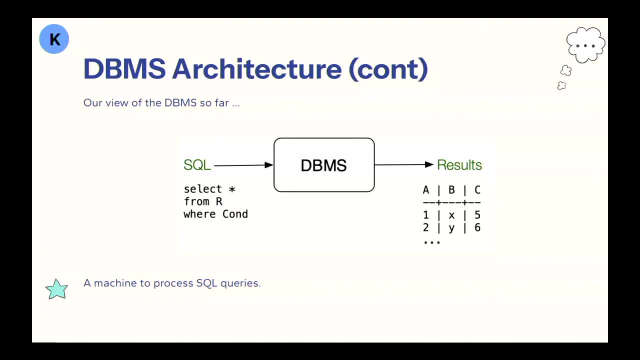 So what we have learned is to use SQL queries and to write queries and give it to the DBMS and get the results, But what we don't know is what's happening inside the DBMS. So now let's learn what's happening inside. 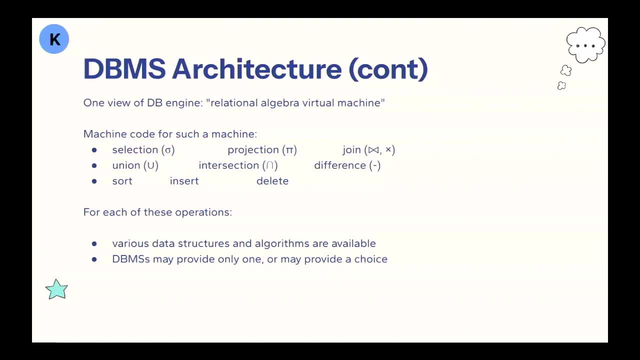 So one view of DB engine. it is actually like a virtual machine for running relational algebra. So if you know the Java virtual machine, so it's actually not executing the source code of Java, It's executing the bytecode compiled from the Java source code. 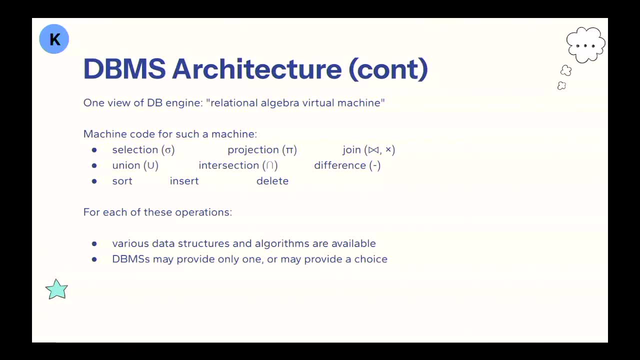 And this virtual machine is like. we can compile the queries into relational algebra And execute the relational algebra operations in this virtual machine. So the machine code of this such a machine is like all the basic operations of what we have learned and some basic algorithms like sort. 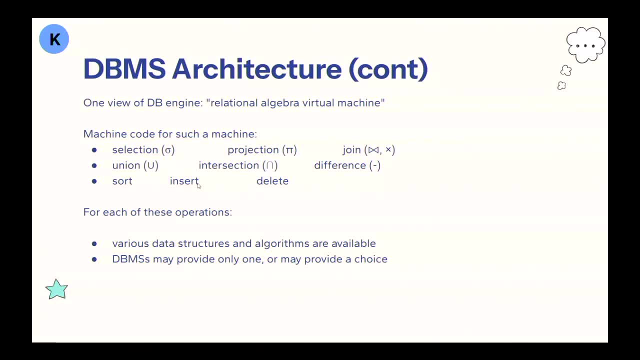 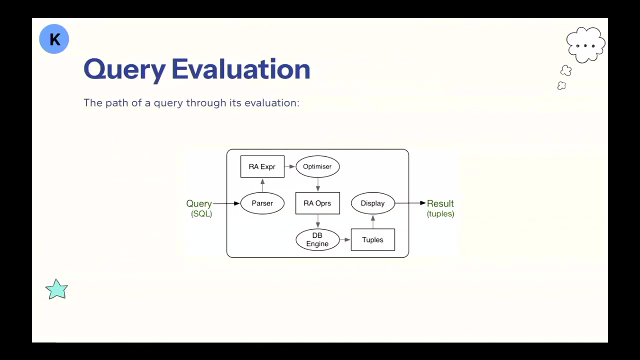 There are some data updating Operations as well, like insert and delete. For each of these operations, there are various data structures or algorithms available, And DBMS may provide only one, or sometimes they may provide you twice. And this is how DBMS do query evaluation. 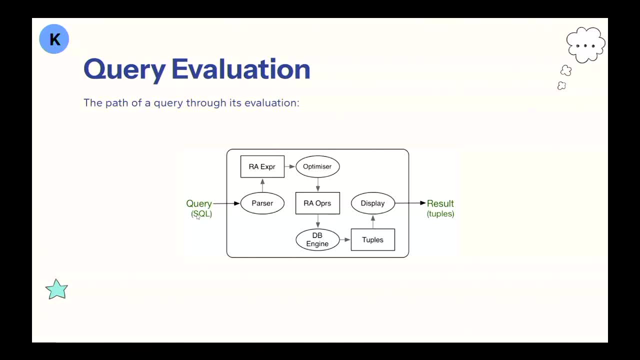 So first It will have an algorithm. So the thing that DBMS will do is it will provide you an algorithm. You can look at the box and the box is the configuration And it's very easy to find. It is very easy to find the information that Citrix. 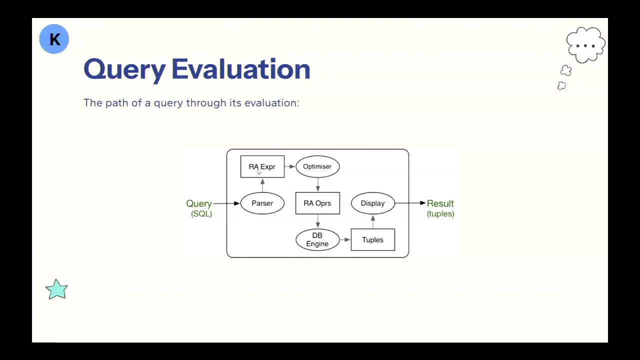 And then you can see that it can be computerized. Another thing that DBMS can do: it is it can run the API. So you can see that in the service you have data, you can do data processing, And then you can simply create the API and write down that data. 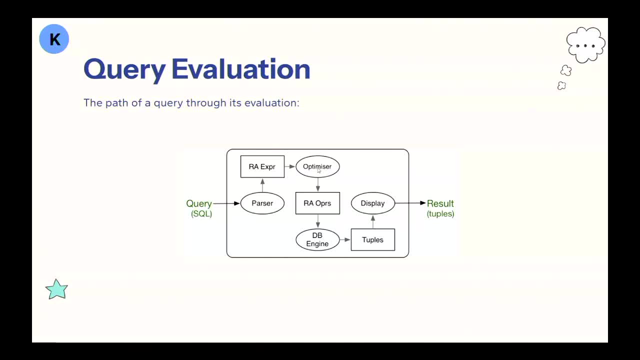 This is actually great for you. You can see the standard data of the software, You can create the API from the database to the debug and it can also do theото delimiter to look for the top nodes of the data And then you can put one order to the data to create the data. 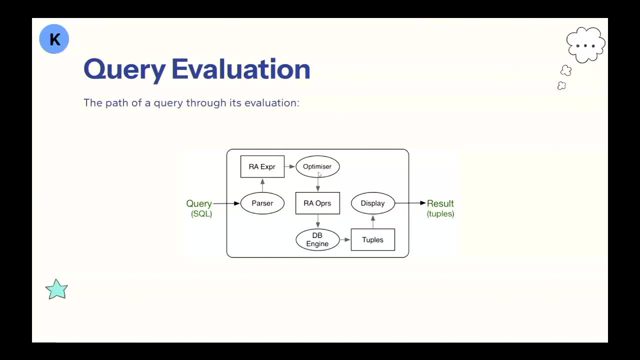 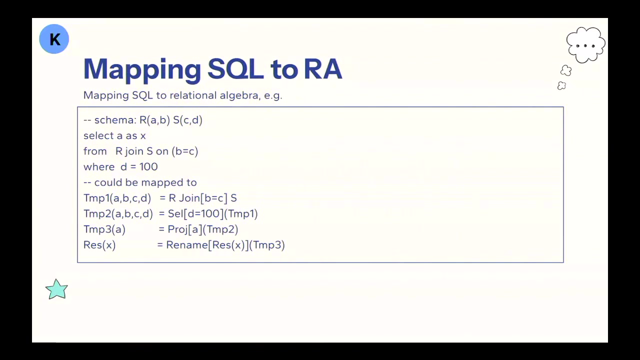 And then you can look for the data, optimize them into the optimized form and and it will supply the the optimized relational algebra operations to the DB engine to collect the total to execute these operations. so this is what's happening inside and, as you could see from what we have learned in our first half, relational algebra has some 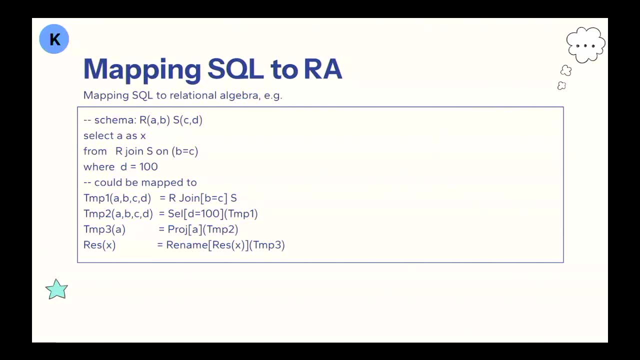 conceptual relation or link with SQL. actually we can map SQL to relational algebra. so actually this is: this select here is essentially the same as these relational algebra operations. as you can see, the the select, select of certain attributes, A is actually correspond to project and the weird condition actually goes to the selection. 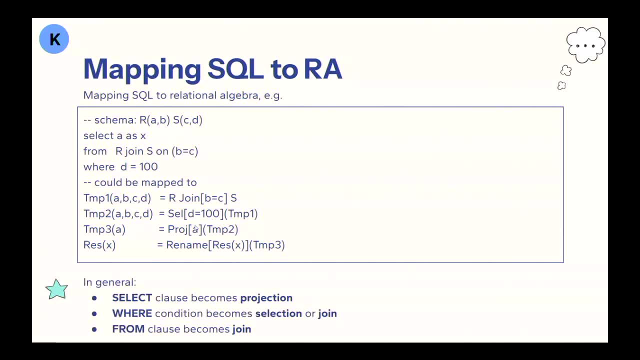 condition here. So the basic mapping here is: select clouds becomes projection, so it is used to specify the attributes we would like to have in our result. tuples And the, where condition becomes selection or join, so it is used to specify the condition for filtering tuples. 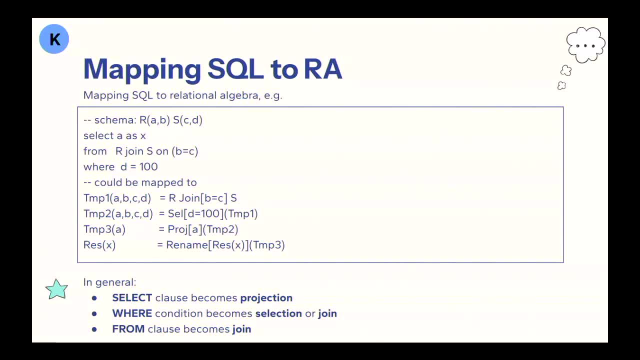 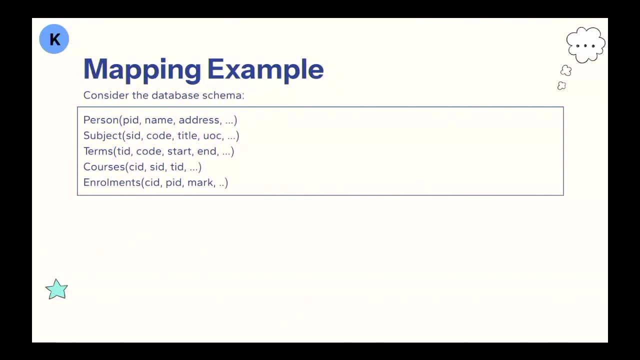 And the from clouds normally becomes join. So let's have a look at an example of mapping here. So for this database schema, we have five tables. We have person, we have subjects. the person refers to students. We have students, we have subjects. we have terms, we have courses. 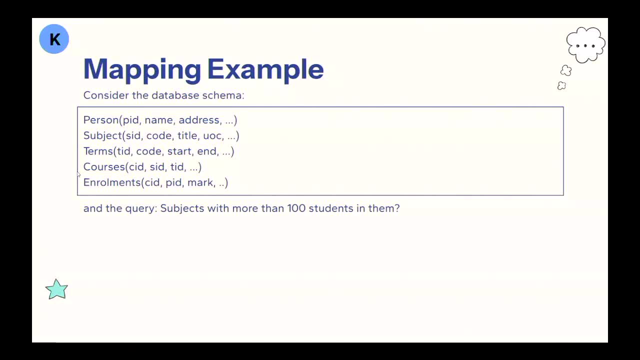 And we have enrollments, And how can we get the subjects with more than 100 students enrolled? So for SQL, what can we do here? Actually, we need for subject. it is not directly related to person. We need to use the relation between subjects and courses. 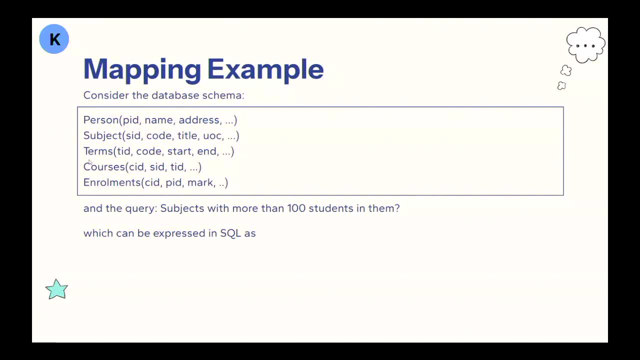 To find out all the courses for a particular subject And use the enrollment table to find out the person, all the students enrolled for a course, And then add them together to count the number of students. So this is what we can do. We need two drawings here, as you can see. 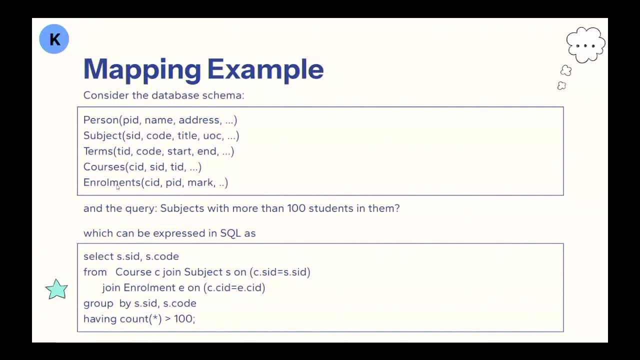 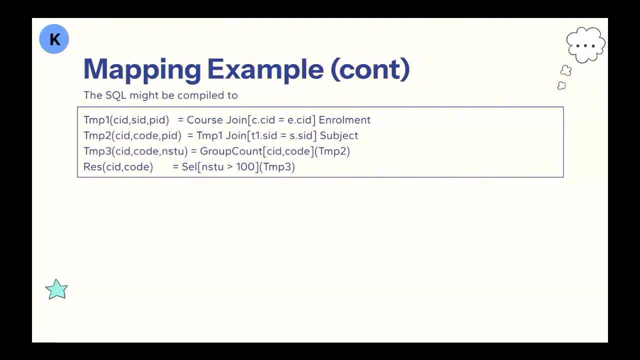 We need to join the table of subjects And we can do that courses, and we also need to join the result from with the enrollment table and this SQL query could be compiled into these relational algebra operations so we can join the two tables together and we can do a group coin, group count. 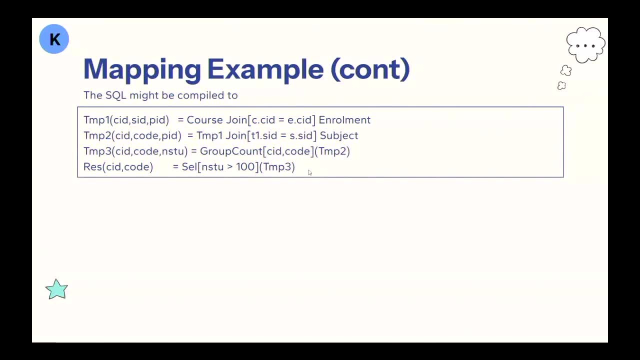 and then we can select. or, equivalently, it could be compiled into this form. so the difference here is: in the first, in the first sequence of operations we are joining the tables, of course, and enrollment first, but in this, in this table, in this result, in this example here, 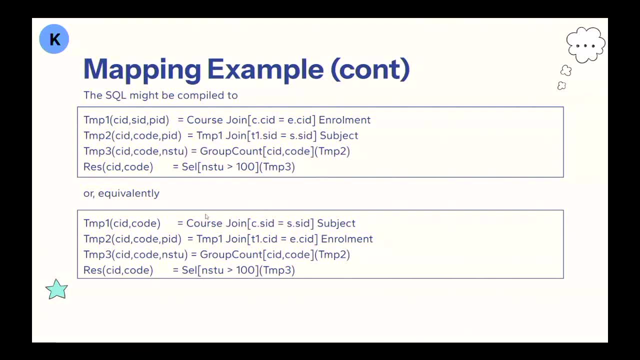 in the second one. here we are joining the tables, of course, with subject first, and then we're joining drawing the result with enrollment these. so the question here is which one is better? so actually the actually for this particular example, we don't have a clear answer without more context. we need more. 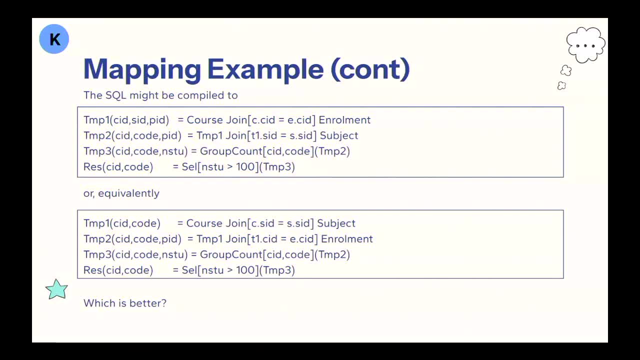 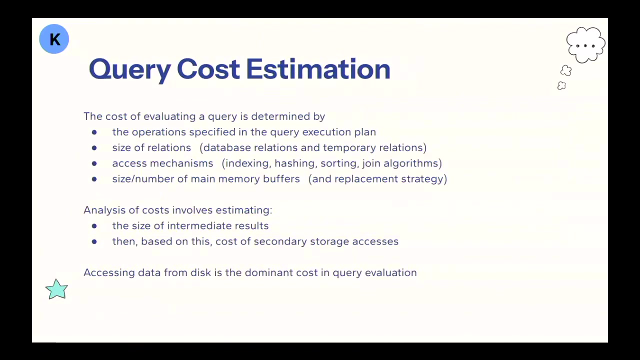 context about the actual data. what's inside these tables to decide which one is better? but? but the question here is: since we can compile the single query into different sequences of relational algebra operations, we need to somehow decide which alternative, or which twice, is better. so that's the the key here. 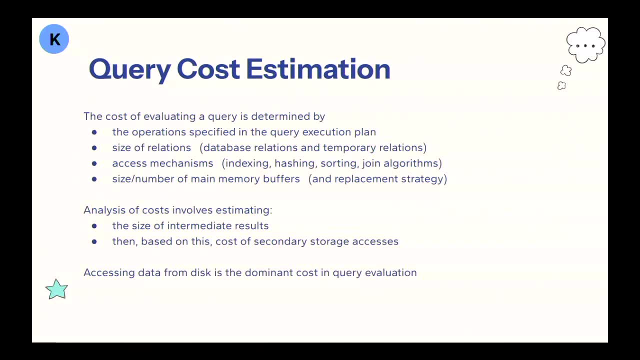 so, and this process is called query cost estimation. so the cost of evaluating a query or executing a query is determined by the operations specified in the query execution plan- and this is a key concept here we will be learning later. and the query execution plan is basically a sequence of 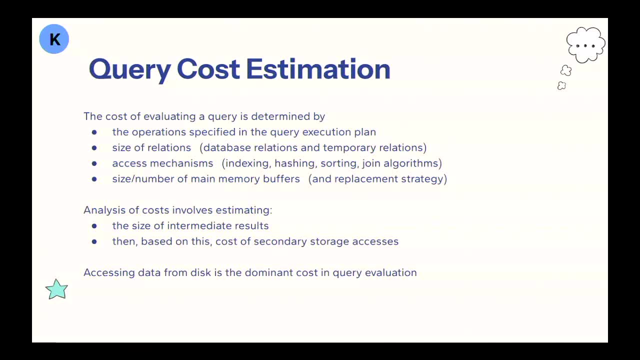 relational algebra operations and it's also determined by the size of relations and it also is also determined by the access mechanisms. if we have indexed certain attributes or certain tables, normally it will be much faster and of course drawing algorithms will also affect the result if we don't use the proper drawing. 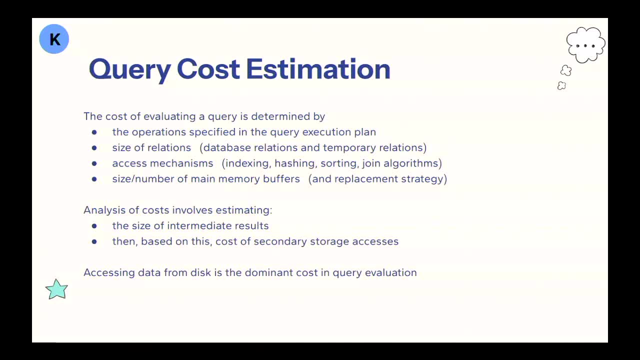 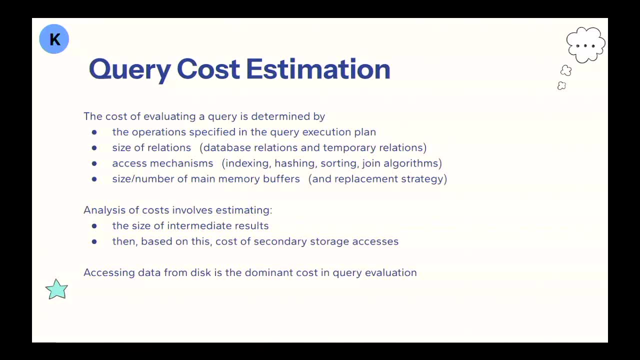 results so. so the size of the intermediate results actually affect the cost of the next steps. so that's why the the just now, in the previous two examples, the cost could be different because the intermediate result of the joining of the first drawing could be different and it could affect the the. 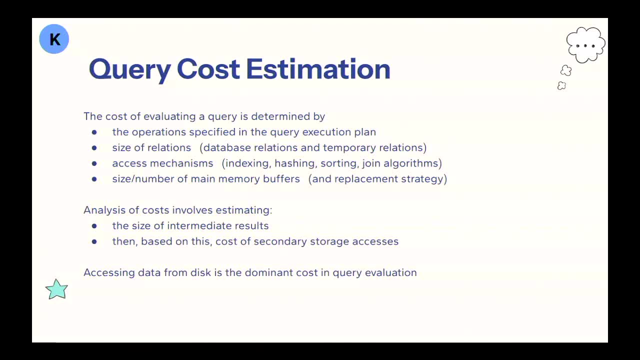 efficiency of the second drawing. so that's why the first step involves estimating the size of intermediates resulting results and then, based on the based on the estimation of the intermediate results, will also need to calculate the secondary storage accesses, because, because database actually stores data under in the hard disks and 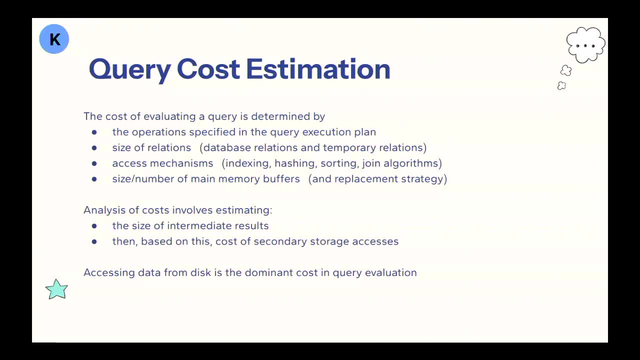 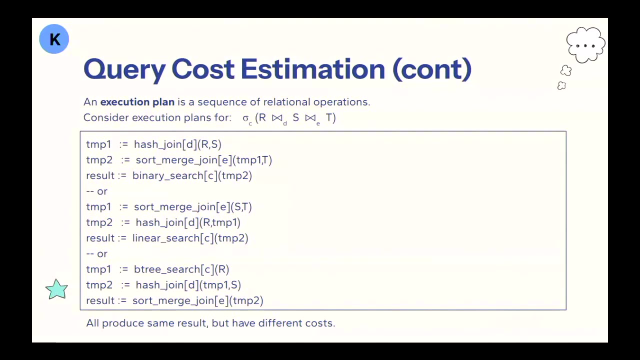 accessing hard disks is much slower than accessing memories, So we also need to take this into account. And just now we mentioned one of the key factor affecting the cost of a query is called query execution plan. So an execution plan is a sequence of relational algebra operations. 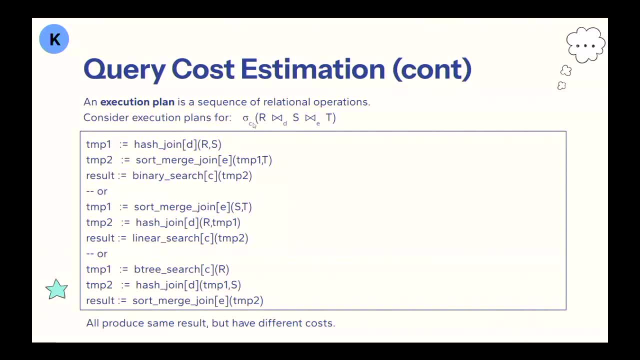 So let's consider this joining of three different tables, the theta join of three different tables on different conditions here. So the first condition is D and the second condition is E, And here are three alternatives For us to do this, to do this query, And they are using different sequences of joining. 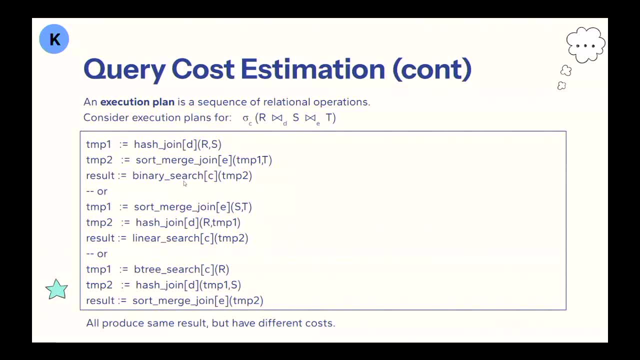 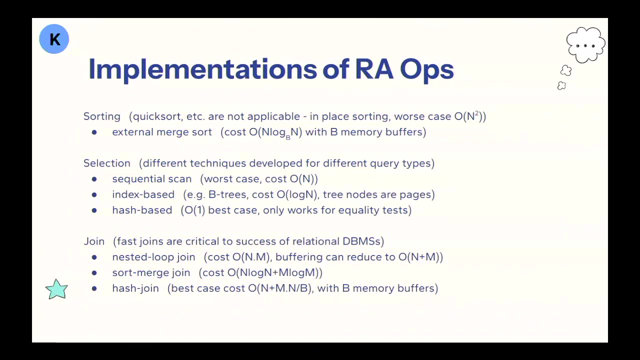 and they could use different relational algebra operators. So the cost would be different. And for an actual implementation of relational algebra operations in DBMS, here are some potential options. So for sorting we can use external merge sort. So note that it's external merge sort We are not using. 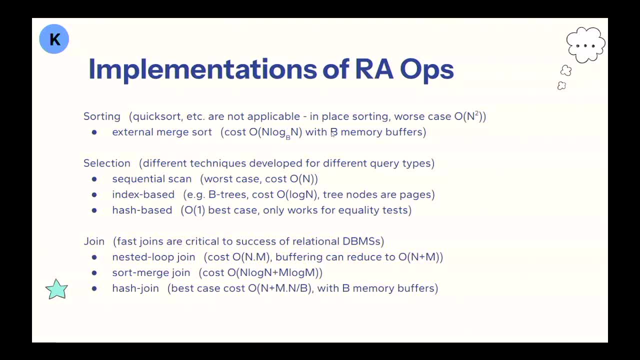 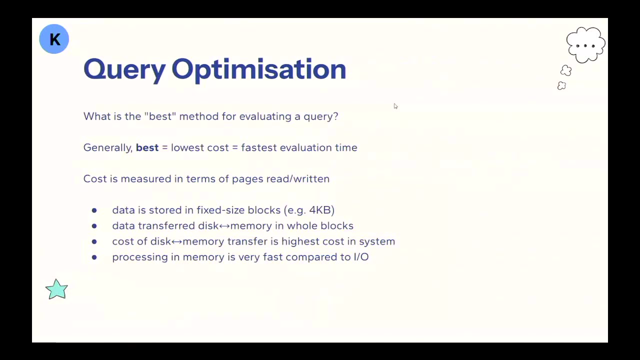 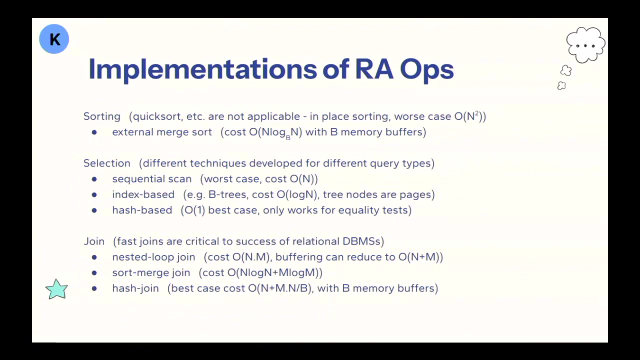 quick sort or other in place sorting algorithms, Because normally the data is stored in the hard disk And if we do in place sorting it will be kind of slow. And the worst case of this quick sorting algorithm is the square of the number of tuples. 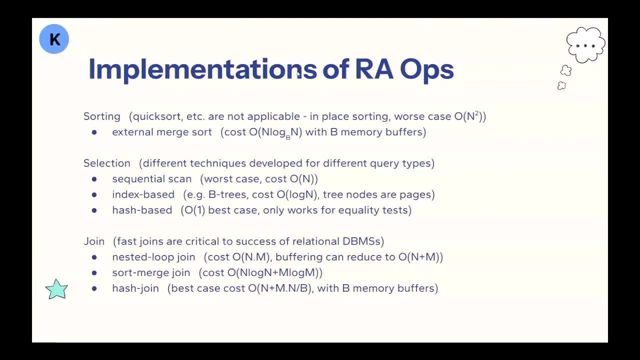 So that's why we should the actual implementation of DBMS. they don't use quick sort And for selection there are many, many different types of selection. So if we have indexed, if we have told the DBMS to index certain tables, 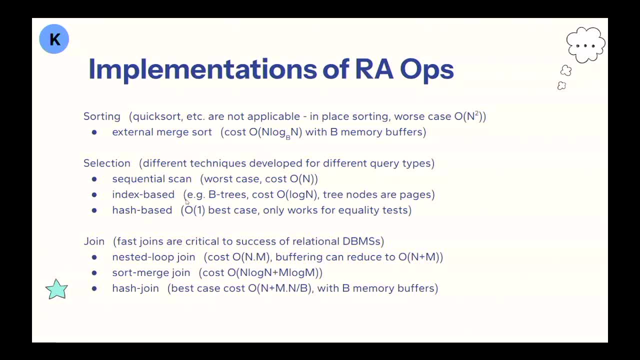 it could use index-based selection Or it could use hash-based selection if it do some specific settings. However, if it don't do anything, it will be the worst case. We will do a sequential scan. We will scan through all the tuples. 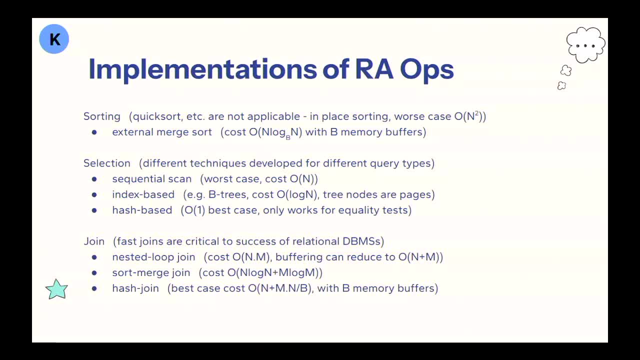 That's very slow. And for joining, we can join tables with nested loops. This is the algorithm we have discussed in the previous slides And this is the slowest one- And we can do salt merge join. We can also do hash join if we have hashed the. 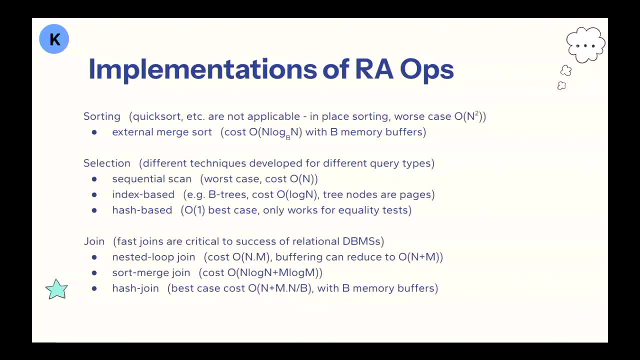 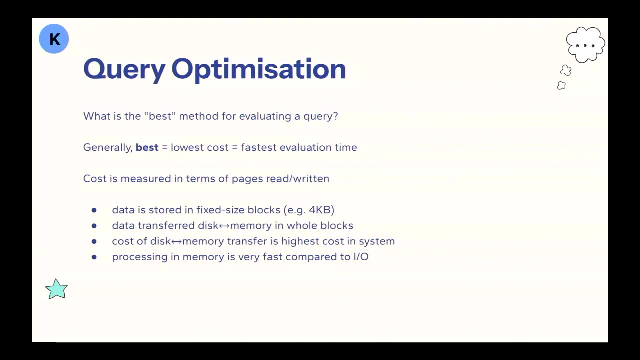 we have maintained the hash table of the actual tables. So all these factors, all these choices of operations could affect the performance here And for query optimization. so we need to decide what is the best method for evaluating a query And generally the best means the lower cost. 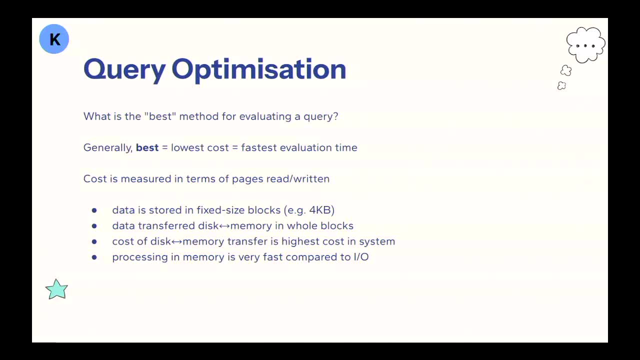 or the fastest execution or evaluation. So the highest cost is the evaluation time And the cost is measured in terms of pages read or written. So it's basically determined by the operations of reading or writing data into the hard disk from the memory and the hard disk. 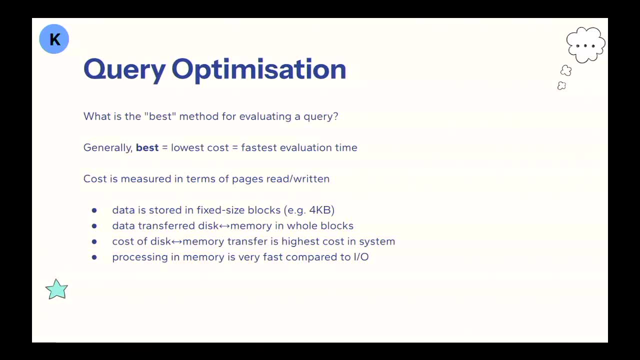 So data is actually stored in a fixed size of blocks, For example for KB, and data transferred from disk to memory is in whole blocks, And the cost of disk to memory or memory to disk operations is the highest cost in this system here. 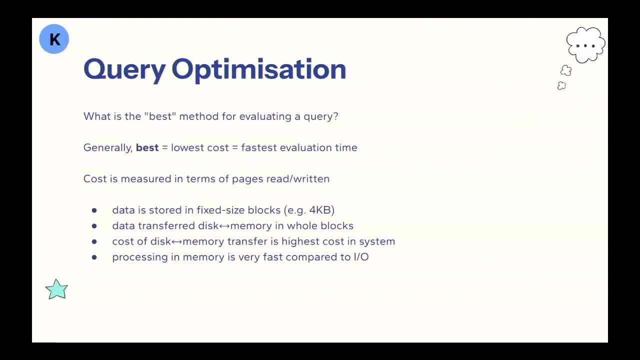 So that's why the cost is often measured in terms of I-O operations, And the processing of data in memory is actually very fast. So when we do query optimization, we should somehow make the DB to avoid interaction with the hard disk. 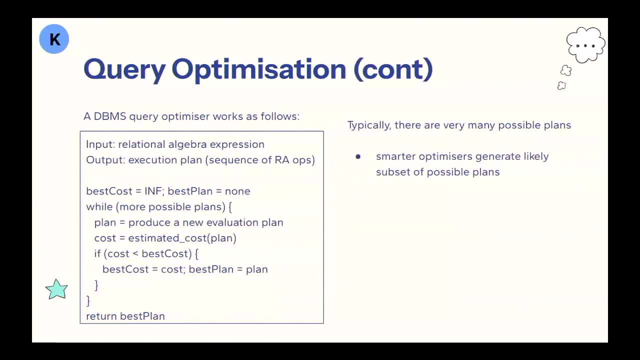 So that's the strategy for query optimization, And here is an algorithm for DBMS to do query optimization here. So the input is a set of relational algebra expressions and the output is the optimal execution plan. So the key idea here is: 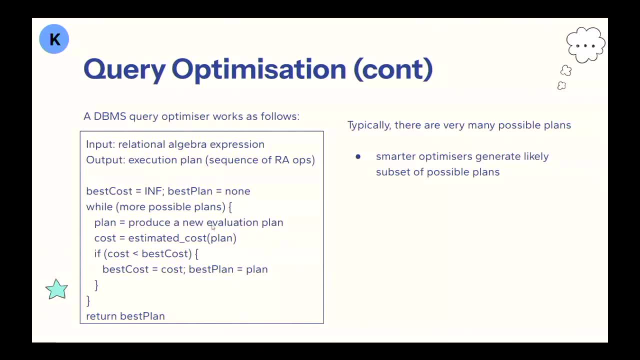 please don't get overwhelmed by this algorithm here. So the key idea here is: the DBMS will just simply go through all the possible execution plans, estimate the cost and select the one with the lower cost. So it's not very complex. 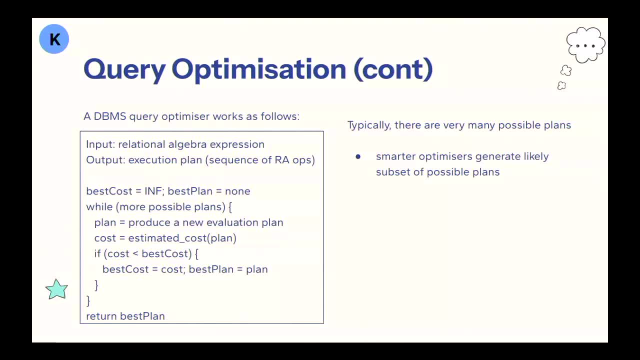 It's just going through everything and select the best And typically there are many possible plans And it's very smart and this optimizer is not actually executing those plans. It's estimating those plans based on their I-O operations. So a smarter optimizer will give us a subset of possible plans. 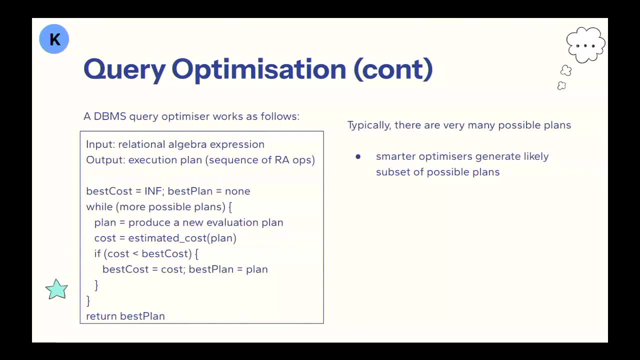 instead of just a single-based execution plan. So that's how DBMS works. So that's how DBMS works for query optimization And that's why we don't really have an answer for the mapping example previously, because we need more context. 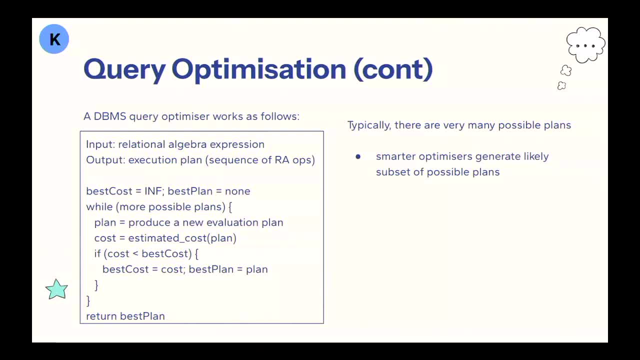 about the size of different tables, about whether they are indexed or not. But this is how DBMS works And you should be, after today's lecture, you should be able to know the concept of relational algebra, how DBMS works and 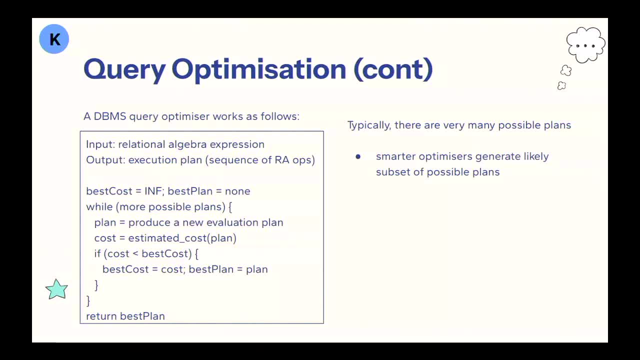 how relational algebra. how are they matched between, how do they match between SQL and relational algebra operations? And you should know that they are useful for optimizing queries for DBMS, And in our next lecture we will learn more, some more practical solutions for optimizing queries. 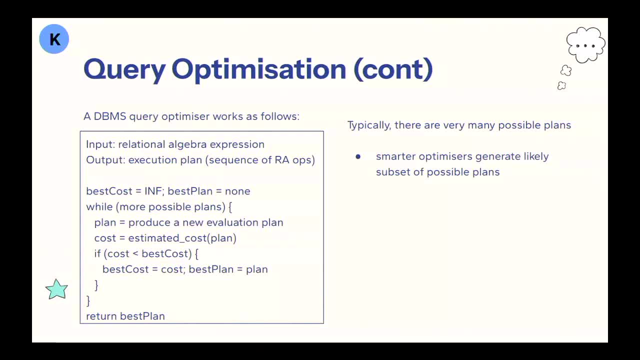 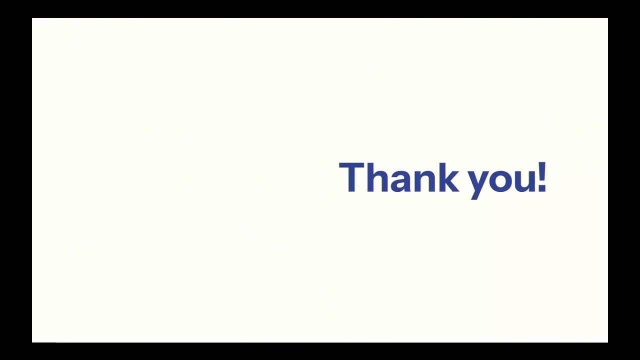 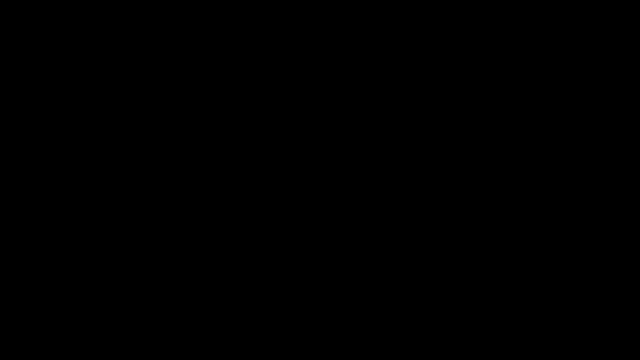 Okay, As a developer, And we will also learn some more features of DBMS, like how do they handle the access of multiple users. And and that's all for today's lecture And thank you for coming. 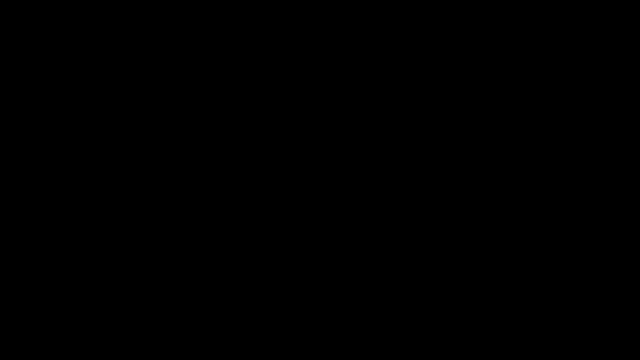